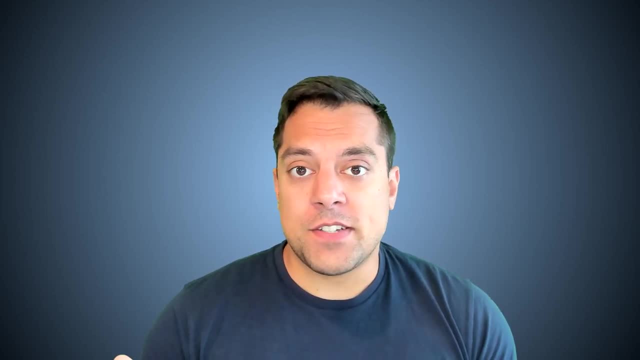 That's one of the goals of a behavioral design pattern: just looking at the behaviors of our objects and how they communicate and achieve their responsibilities. And the specific behavioral design pattern I'm going to be looking at is called the command pattern, And this goes by other names, so sometimes you might hear it as the action or 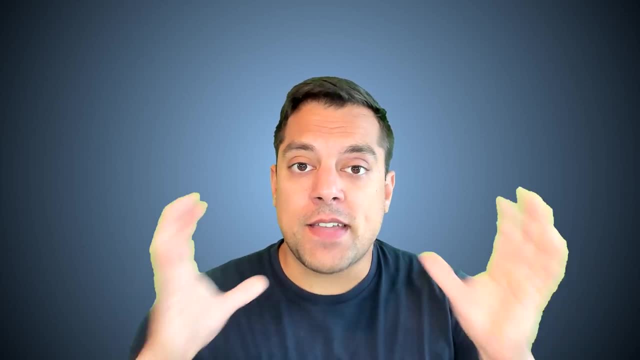 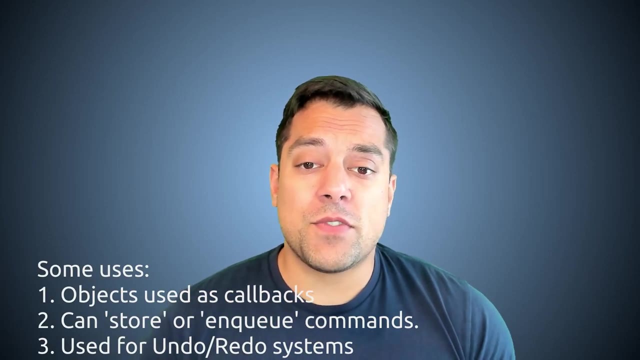 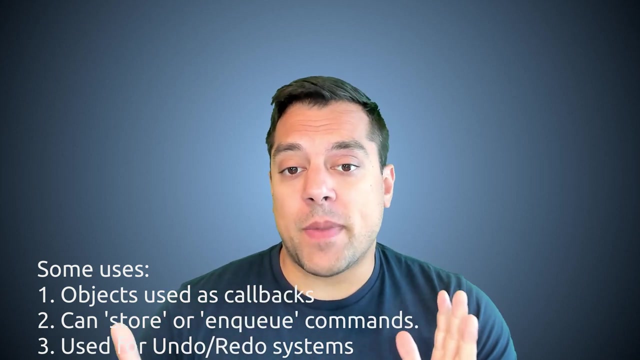 transaction pattern, But basically it's a way to take objects and model them as commands that execute actions. So the command pattern can be useful in a way to have object-oriented or objects put together and used as callback functions. You can use it to model objects as commands. You can use it to model objects as commands. 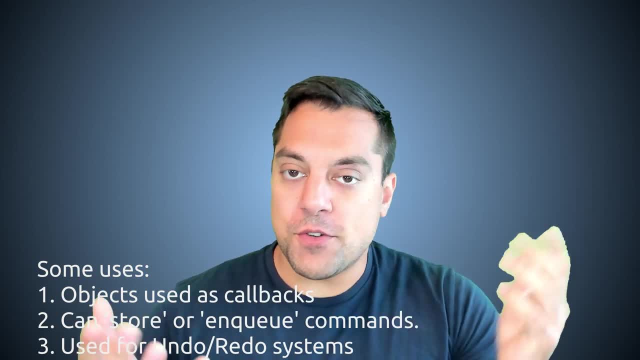 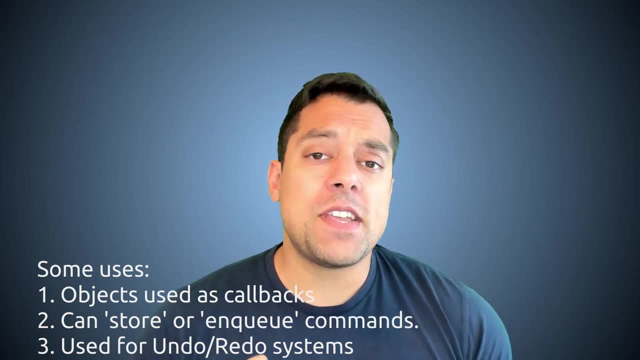 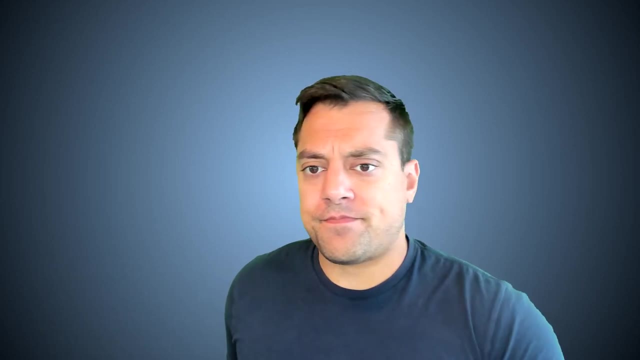 And it's also useful for things like building undo and redo systems. We'll see a way to do this in our example today And we'll go ahead and get started in a moment, But before we begin, I just want to bring attention to two books that are going to be really useful. if you want further, 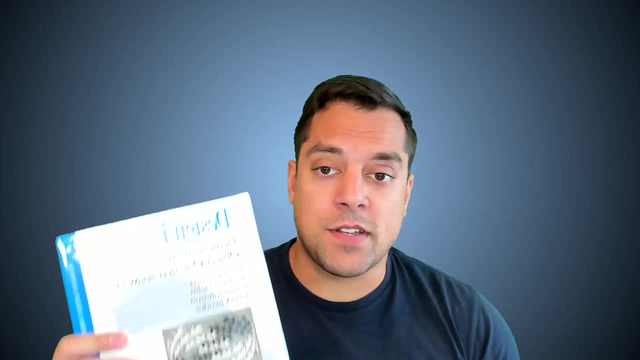 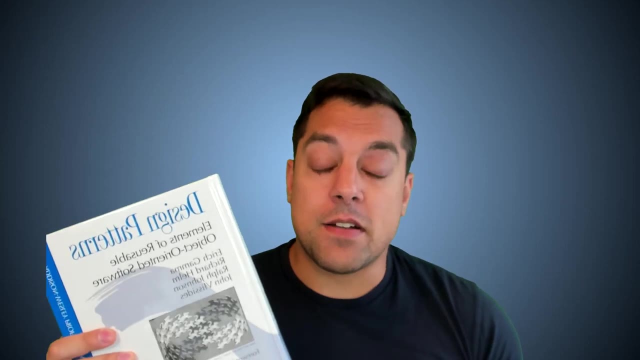 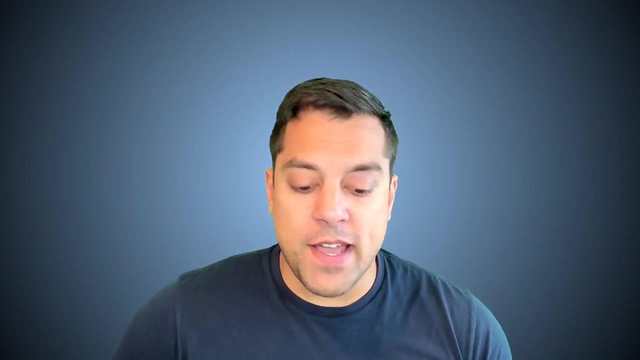 resources and all the sort of nitty gritty implementation details. So the design patterns book, also known as the gang of four book. It's an excellent book for reading about the band pattern as well as many other popular patterns. And another very useful book is known as the game programming patterns book. So this book here is. 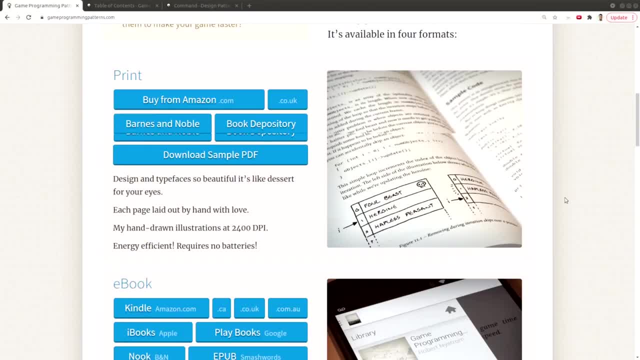 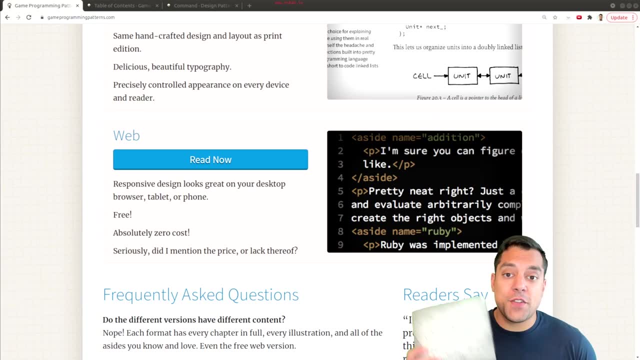 written by Robert Nystrom, And it's actually a free book here, So we can go ahead and read it from the web. So, again, with that said, this is a free book, But I do have to give credit where credit is due, And I have purchased this book because I really think it is a great book And I 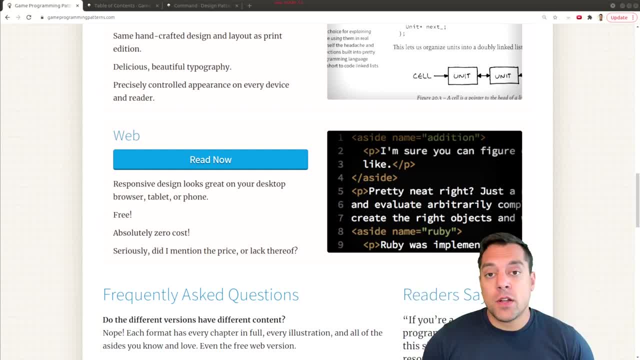 have purchased this book because I really think it is a great book. It's a testimony to the author for doing a really nice job writing the book and supporting them. I'm not sponsored or anything, but I just wanted to throw a shout out there because this was a very useful book for me to 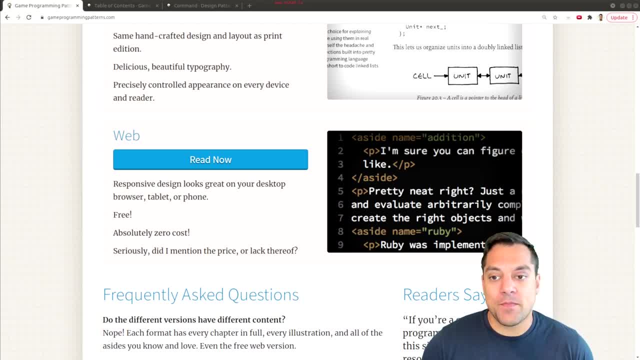 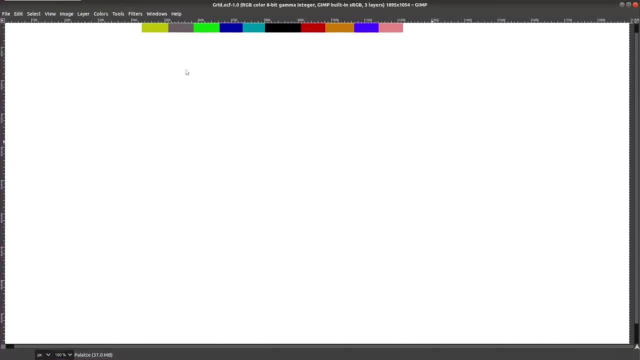 learn some of the design patterns and have two resources to look at. Alright, so, with that said, let's go ahead and dive into the command pattern, And before we dive in, though, let's just try to understand this pattern a little bit. Okay, so I'm going to go ahead and switch to the drawing board. 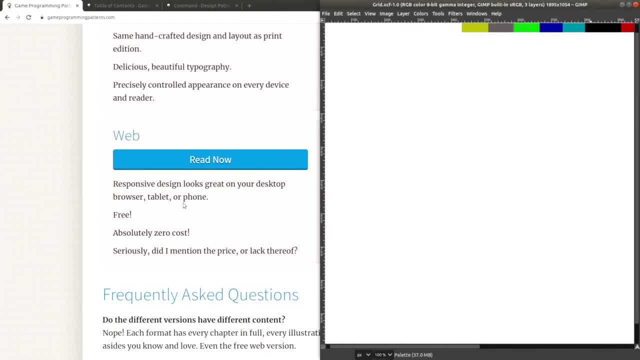 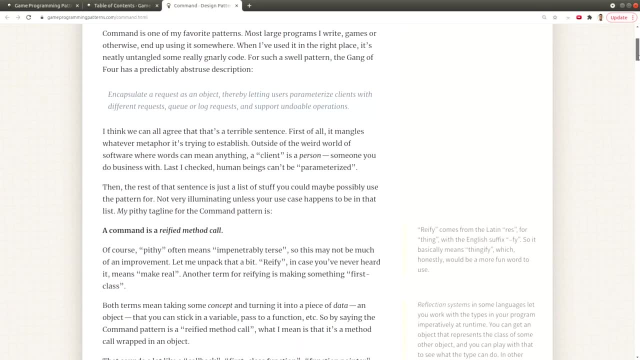 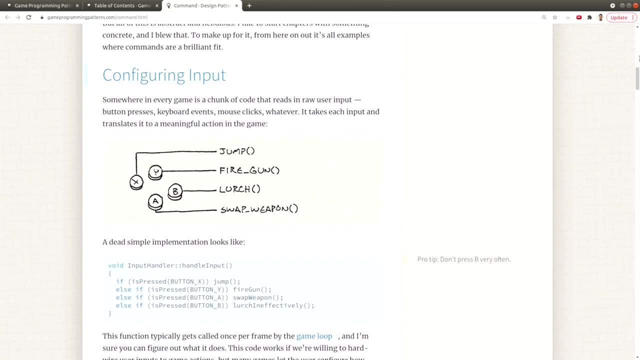 here, just so we can understand the pattern, And if you want, you can go ahead and take a few moments to read in the text the command pattern here. This is essentially what I'm going to draw out here And I'm going to use a similar example here of modeling different commands as button presses or 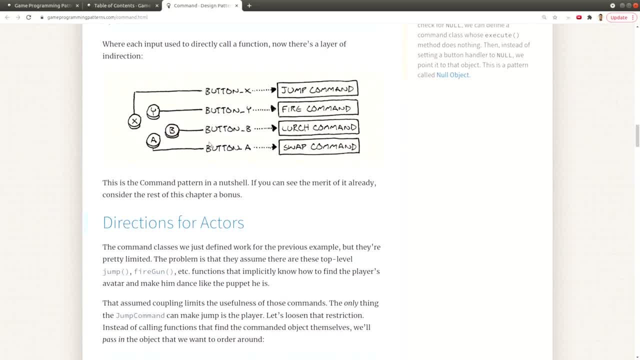 commands on, say, a game controller. So there's a nice illustration here where Nystrom, the author of the game programming patterns book, is modeling commands When you press the X, Y, B or D buttons or a button to do some sort of function. But rather than having a specific function, call we 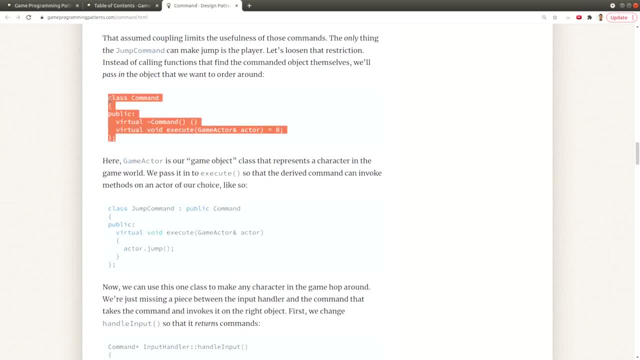 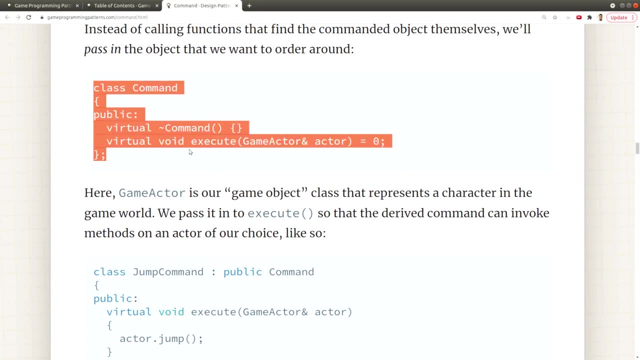 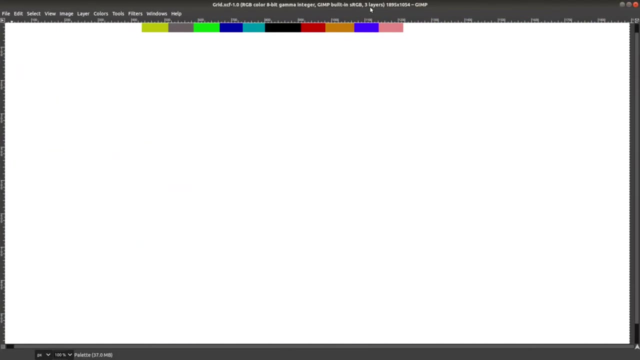 encapsulate things in a class called command and then execute those actions here, Okay. so there, it is just a little bit bigger here, Okay. so again, let's go ahead and just illustrate what this allows us to do here. So how I'm going to approach this problem is again, let's say, I have some sort 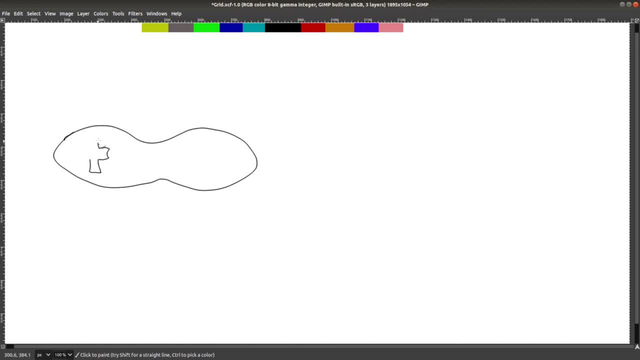 of you know game controller And I'll draw it like this. you know maybe an old school on Nintendo controller. whatever, we've got our buttons here And you know four buttons here, So when I press this particular button here, 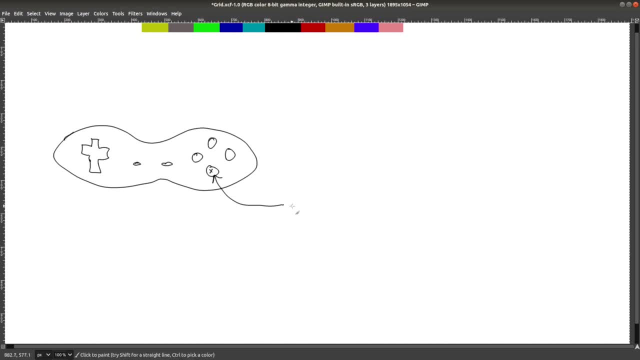 and let's say it's a PlayStation controller, so I'll put the X there. we want some command here Now, depending on what the game is, maybe this is a jump action or maybe it's an accept action. if you're looking at a menu or enter, right, and we have these various commands. 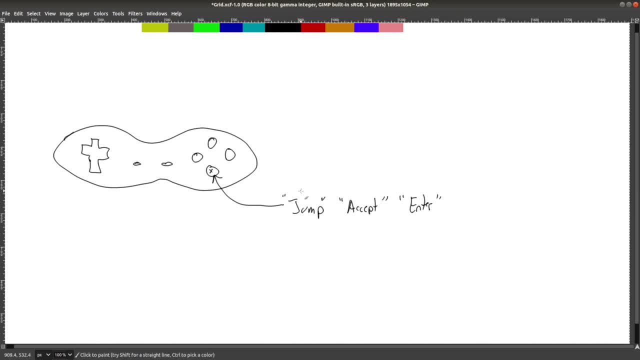 depending on the context that we're in. it would be really useful if I could wrap all of these different actions or commands into a common class, So I could say each of these are a type of command here. So if I just sort of draw this as an inheritance hierarchy here, all of these different 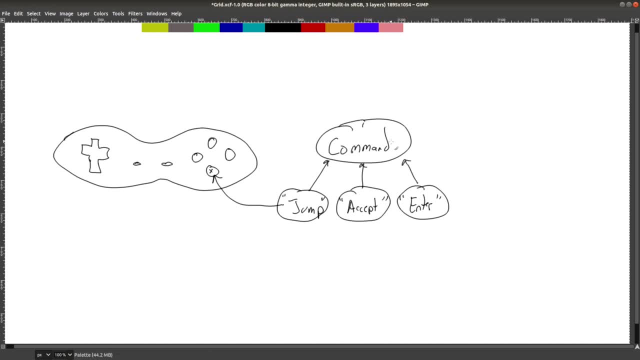 commands would inherit from one common class, And that way my x button can just accept one of these commands here it doesn't matter. So I can just sort of model this for example: command- And let's just make this a pointer- x equals. 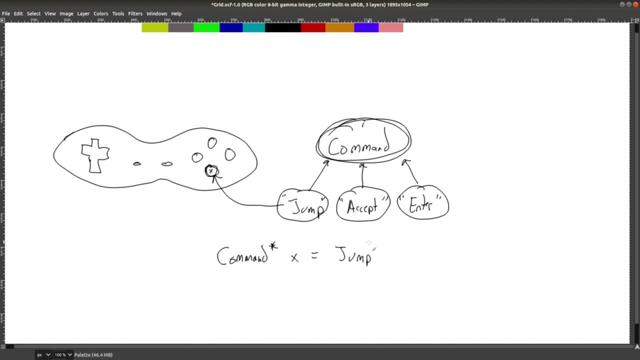 you know some other type of command here. maybe it's jump action or whatever you know. we've instantiated this as okay, so that's the basic idea here. Now, what makes this really powerful here is that, since I can encapsulate things into objects, I can perform actions on. 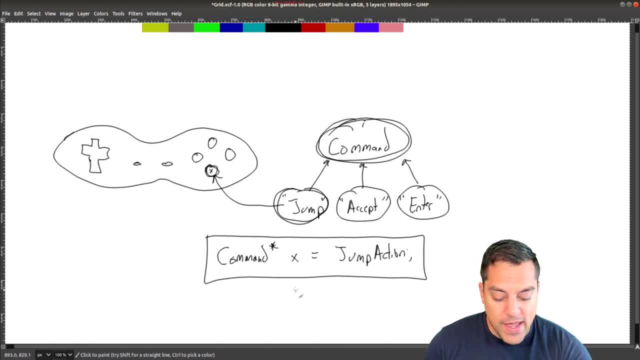 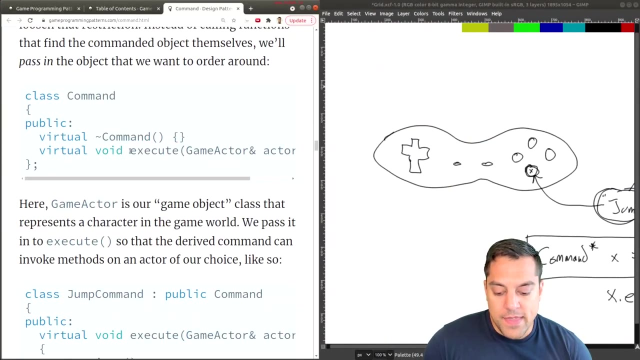 them. So, for example, I can just now have the x dot execute, for example, which would be a member function of this command class here. So let me go ahead and just illustrate that and point that to you in the nice drum code that every command has or must have an execute action. Why must it? Well, in C++. 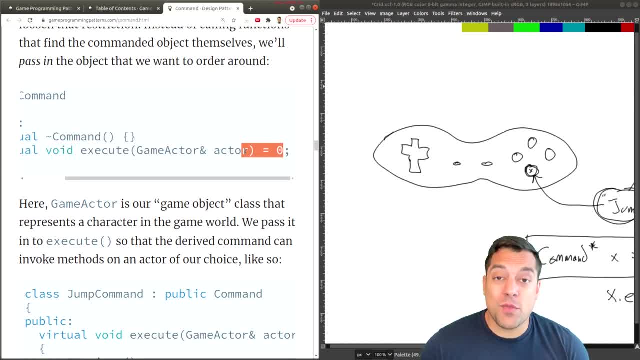 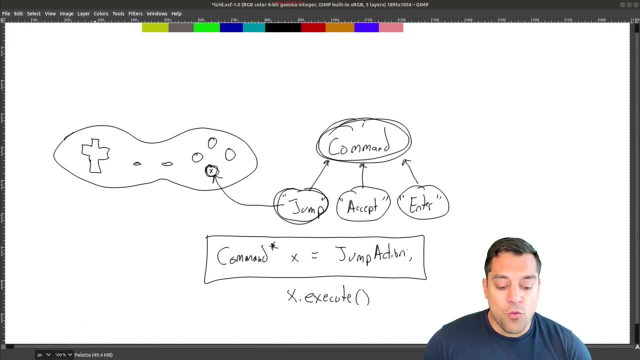 when we have virtual void and assign something to zero. we call that a purely virtual function, so it must be implemented. Okay, so that is to say we must in our jump command, implement, execute this member function here, And likewise for accept or enter or any other amount of commands that we have. we can. 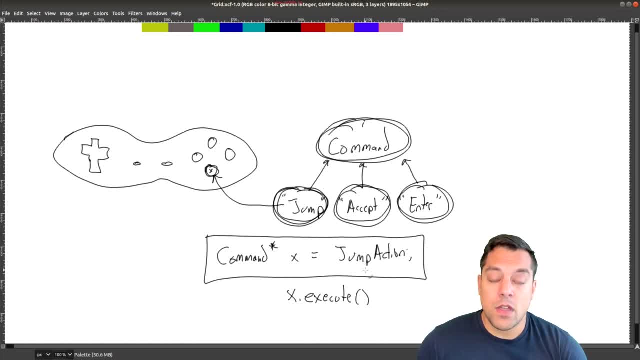 we must rather implement the execute function. Now, what also makes this very powerful is, since we've encapsulated everything, or everything is a type of command- we can actually delay or control what we actually execute. So, for example, we could immediately, when I hit x, say: okay, call. 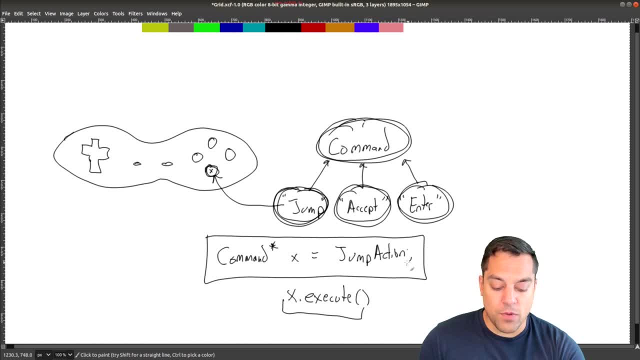 you know, whatever the appropriate member function is for this variable here, So execute, which happens to be some sort of jump command. But I could also delay that and queue these commands. So maybe I have some data structure here Or I have some, you know. command one: command to command three, command four, command four, five, six, all kinds of command that can actually cycle. but I could transfer it right here instead of by say, okay, j, And when we Polygon of the function is right over here, I'm going to generate this variable ten and no within the. 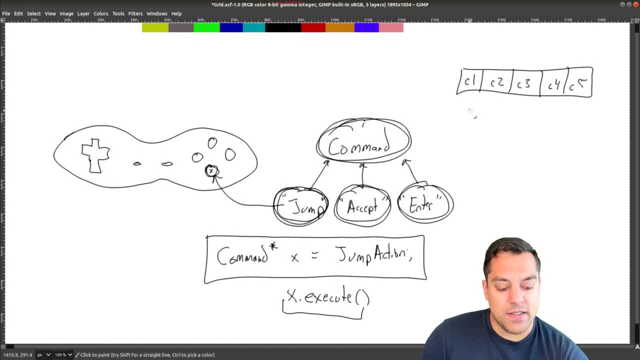 갶습니다 of family say okay, when I called to like to specific entity here. whenever I do, I can create some Genau five, etc. So that's the idea And these are all commands Okay, and maybe we have some sort of. 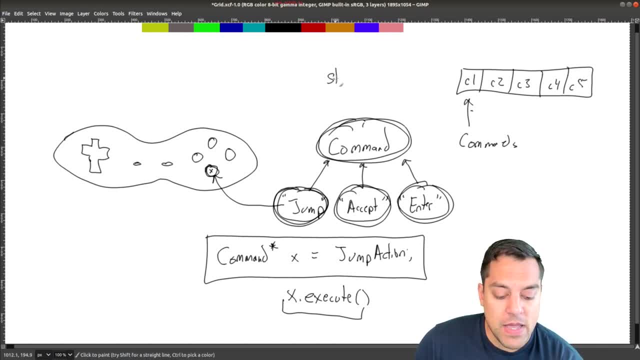 data structure, maybe it's a queue, maybe it's a stack, Maybe, you know, in C++ we like to use vector, So I just have a vector of commands here, Okay, and maybe these are pointers or whatever. Again, we probably want to be a little bit careful storing a pointer here, But But that's the idea. 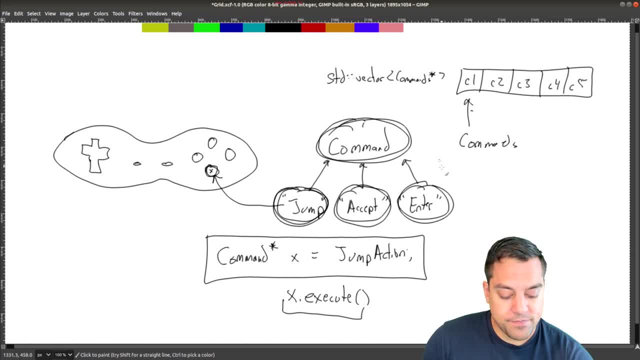 that we would have each of these commands here. Okay, so then this would look like C one, call your execute function, and so on. Now, the last thing I'll mention before we do a little bit of live coding is not only can we enforce that we have an execute command, but we can also have 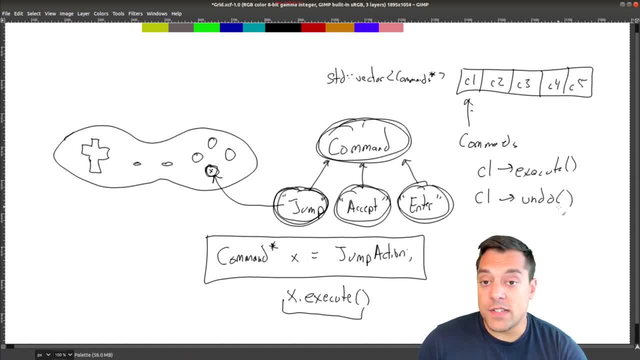 C one and then implement undo or any other associated command. So in a sense I'm able to walk through this command structure here of vectors and execute all the commands. But I could also walk through this structure here, which happens to be a vector in this example, and undo all the commands And the 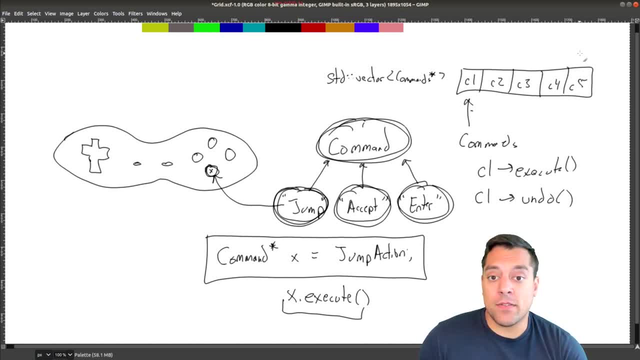 user would implement whatever the opposite of jump is. So maybe you know not jump or return to your previous position or whatever. In the context of a word application, for example, where you're highlighting text and you're maybe you delete something, you could implement an undo action which returns that text right. So 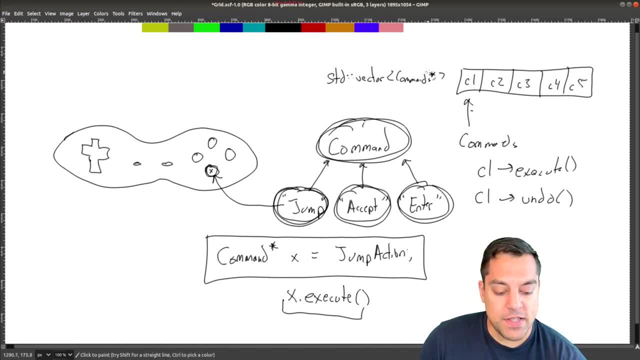 you have this history of commands here, So I might call this history here With our vector. Now you'll have to think a little bit about how to implement this. It's actually a common homework problem, So using perhaps stacks and undo and a redo stack might be a hint as to 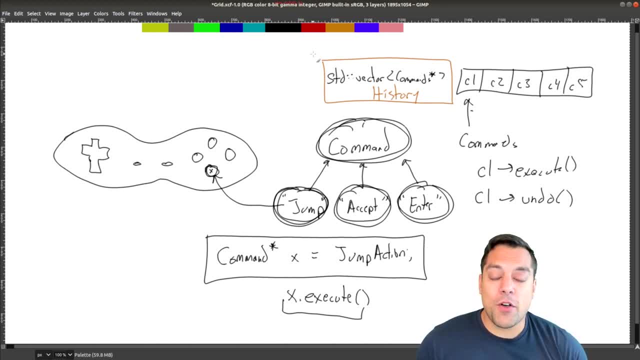 something useful to do. Okay. so where I want to go ahead from here is just do a little bit of live coding, Now that we sort of understand the pattern or how to model it, And let's go ahead and see how we can do things and C++. Okay, so I'm just going to shift things over here and open up our window. 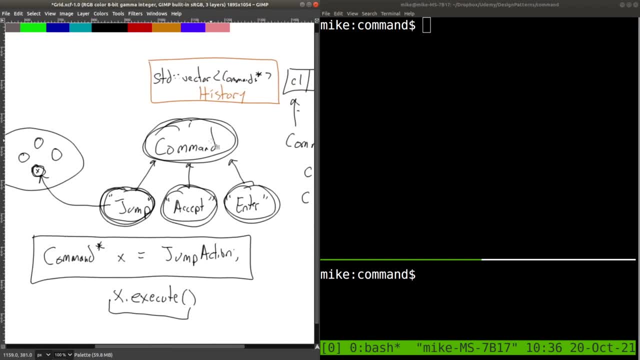 And again, here's a little reminder of what we're trying to achieve And I'm just sort of focusing on this higher key for now. So I've still got a little bit of a blank space that I want to give that back. So I'm just going to go ahead and give it a new feature And I'm going to go ahead and put it down a little bit. 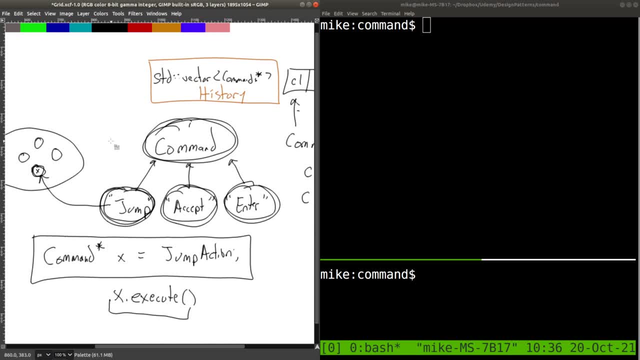 And I'm just gonna give it a name, And then I'm going to give it a little bit of a name And then I'm going to go ahead and edit it out of the, for now, this command hierarchy And, if you want, when you're programming this, it can be a useful 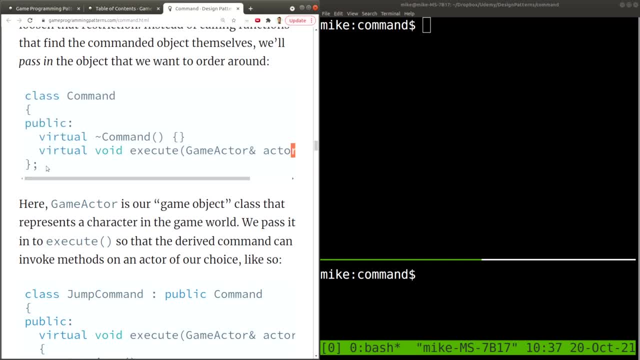 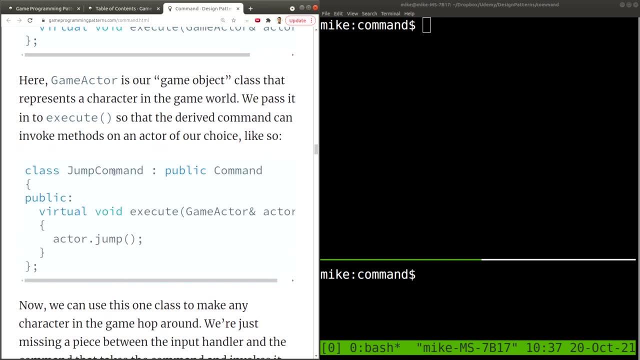 reference to also look at the Nystrom book if you want a good online resource, just to see the command pattern here and what we're doing here. So this idea of what's going on with, say, a jump command here, Now let's go ahead and create a source file here And I'm going to go ahead and 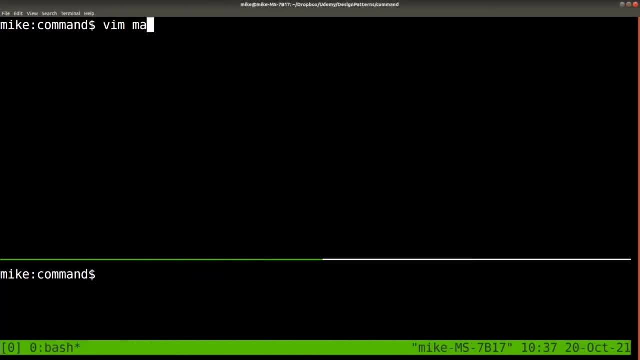 make this bigger here, just so you can see all the text here, And I'm going to do this all in one maincpp file. Of course, you'd probably want to abstract these into different files, But for the purpose of getting everything on the screen at once, I will do this here. So we need some main. 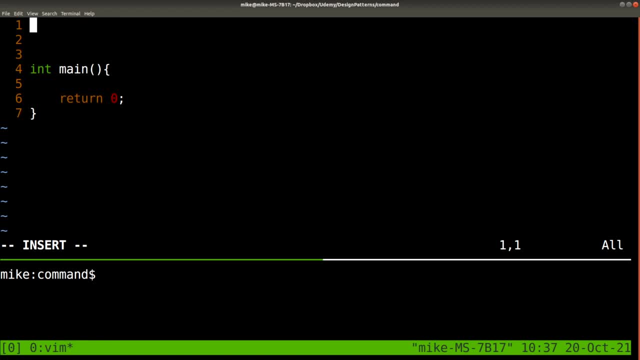 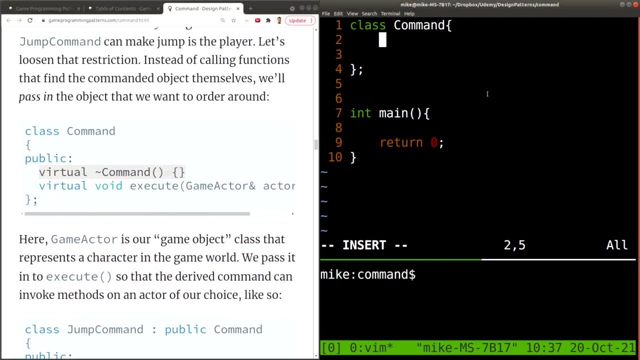 function here and return, and we want to create our command class here. Okay, so this is going to be our main class here, And what we're going to do is again create a, because we're going to be using inheritance. we want to use a virtual destructor. 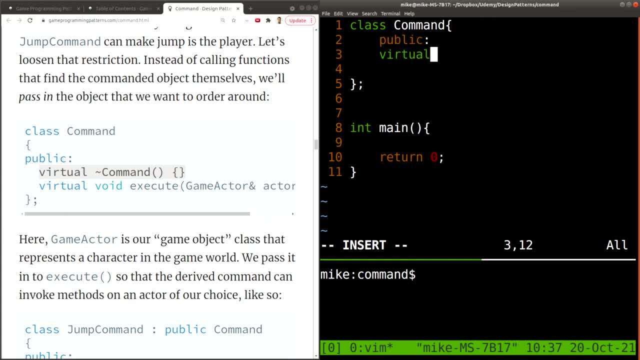 here. So this needs to be public- And our virtual destructor, And for now it's not going to do anything. And then the key is that we have a virtual void execute- And I'm going to model this a little bit simpler here- And this must be implemented by any class derived from command. 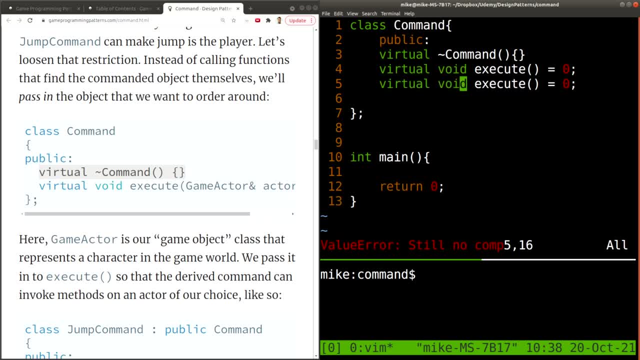 Okay, and I'm going to go one step further and go ahead and give us a undo function which would be the responsibility of any class that's derived from command. to also implement an undo function which we'll say is the opposite of whatever execute is Okay, All right. So what should we do for our commands here? Well, let's. 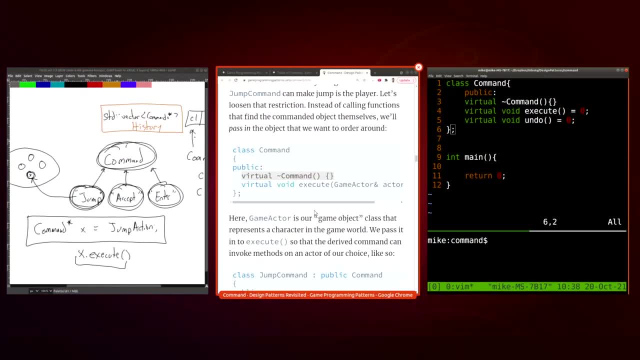 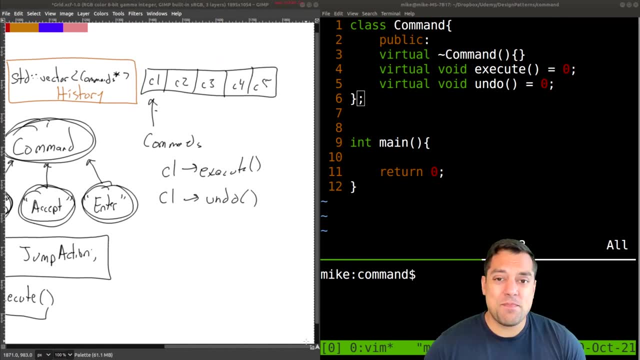 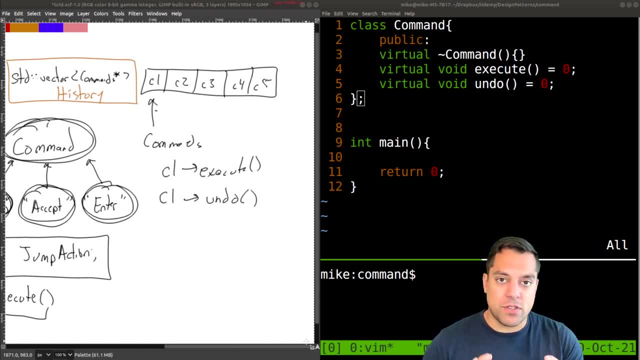 model, the simple case. sometimes there's multiple ways to do the design patterns, but just to get something working, try to draw it out and understand what's what's going to happen. so in this window down here I just want to illustrate. maybe we have some game in here that we're trying. 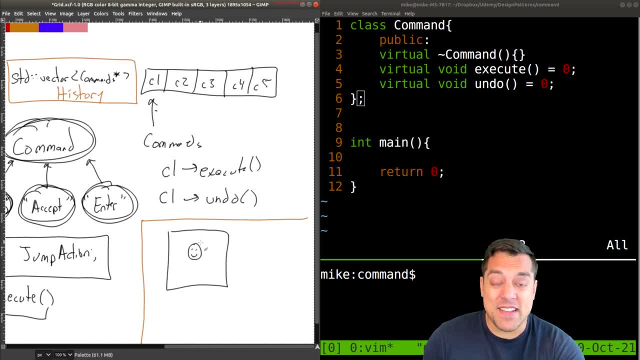 to model And we have some character here And they can sort of move around positions here. So the left to the right, Let's say, if there's a link in here to Google Analytics or the, do recognise the topic here. just do the sort of cooked powder. 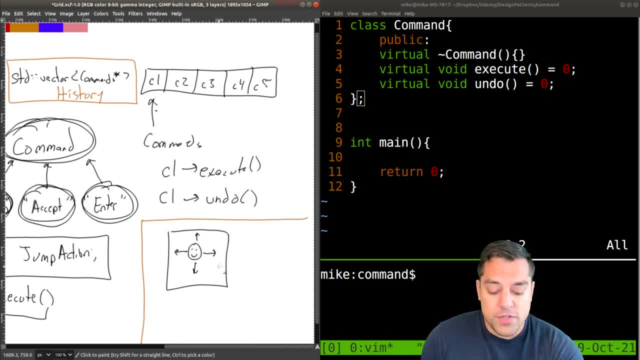 you know, up down, whatever, And we want to store those positions as x and y positions. Okay, so this seems like something reasonable that you'd want to do in a game, And so for now, let's just model some action of moving, Because eventually, what I want to show you is that we can. 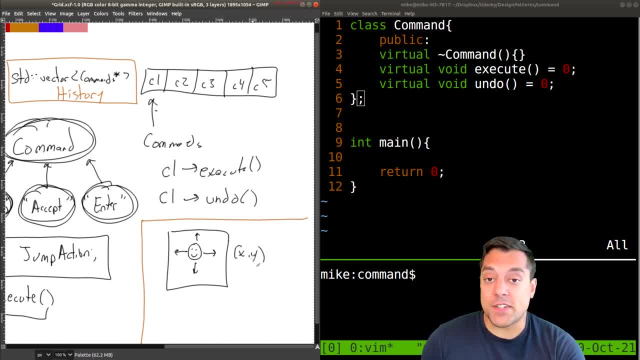 queue up these requests in some vector. these are going to be our sort of move commands that take place and then be able to move or traverse through this data structure, perhaps undoing the move actions. Okay, so now that we sort of have a concrete idea of what we're trying to, 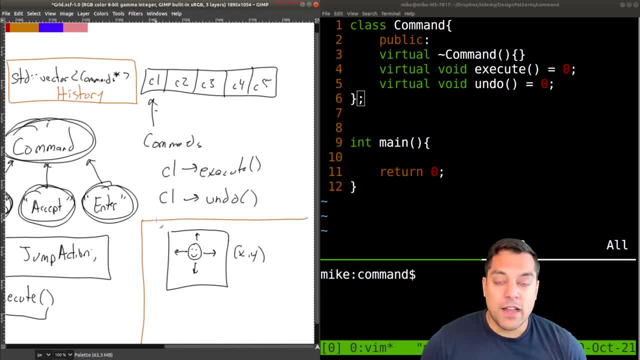 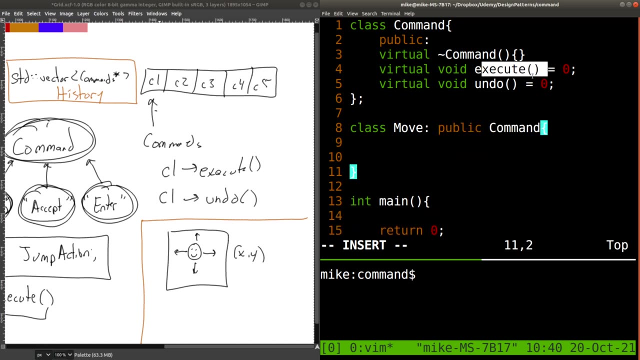 achieve just some command where we can move a character around, let's go ahead and proceed. Okay, so let's go ahead and implement a class here: move, And it's going to inherit from command. So that means again that I must, I absolutely. 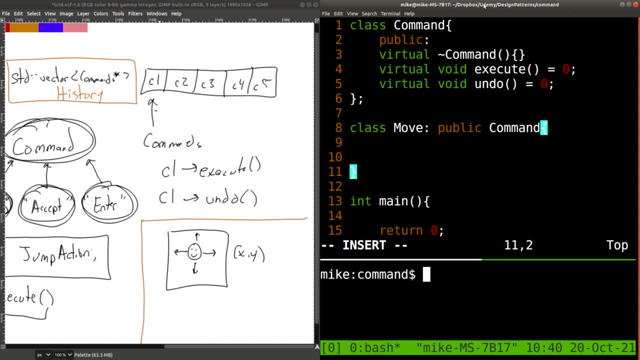 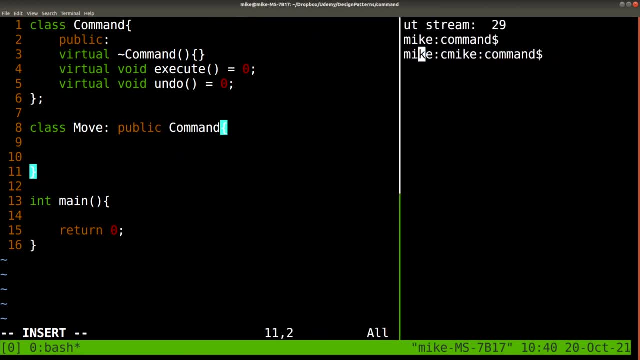 must implement these functions here And I want to go ahead and just demonstrate that by trying to compile the program here at this point. So you should see a bunch of errors at this point if you're following along. So if I do G plus plus, I am using more modern. 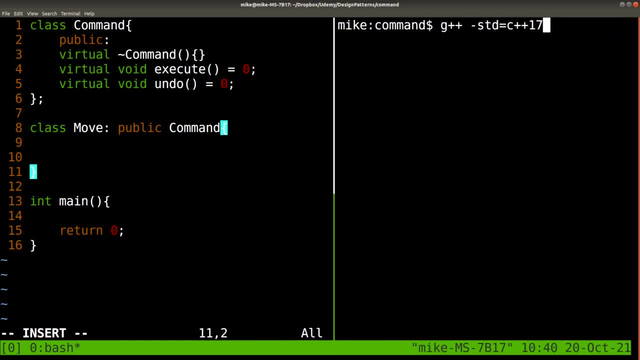 C plus plus these days, So I like to always compile- and C plus plus 17. And this is the main program And let's just give it some output. So be the product program. Okay, Oops, and let me make sure I save here. Okay, So one syntax error, missing semicolon. And if I try to compile, 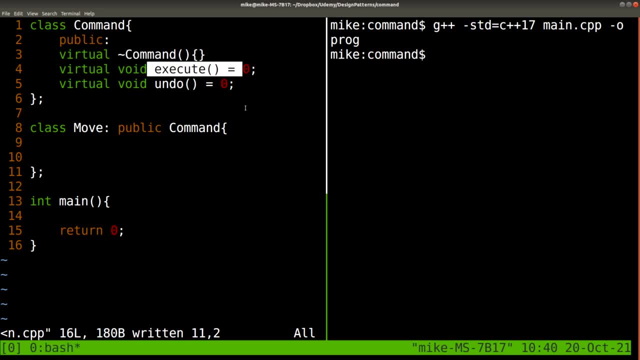 actually it's. it's pretty good here. I guess we don't have any complaints here. Now we do have to use this. So if we try to instantiate this without implementing these functions, we are going to have a problem here. So if I try to just create a move command, 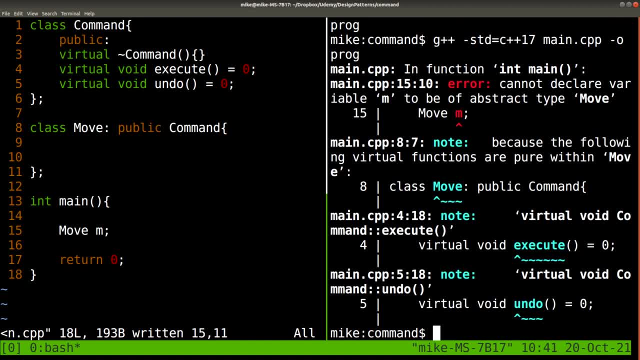 here like this: let's see what happens. Well, now we get our command, So we're going to have a function right like a little code here, And then we get our function. And then, if we start on the new function, we're going to be able to get the function of the new function. So let's. 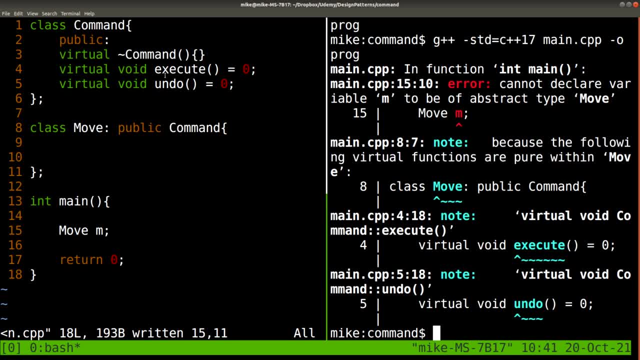 just let's just do this And then let's actually do this. So we're going to say starting to execute here, we're going to give it like that. Okay, so now we're going to add another code And we're just going to continue this, giving ours a new function because we received the 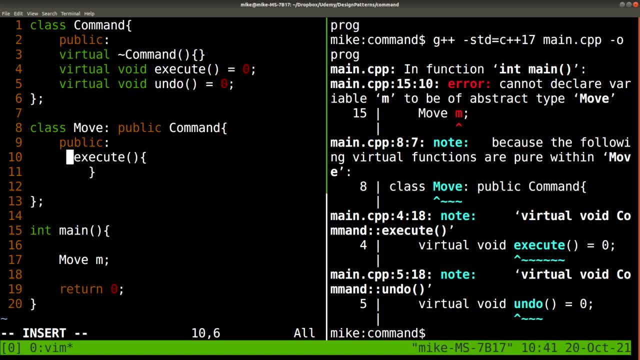 address which in the compiler? the compiler is the one that will give it a GrooveUpar. are all the errors here? The compiler, the newer compilers, are smart enough to say: Well, if you never use this, we won't give any errors. But again says: can't declare variable M of abstract type. 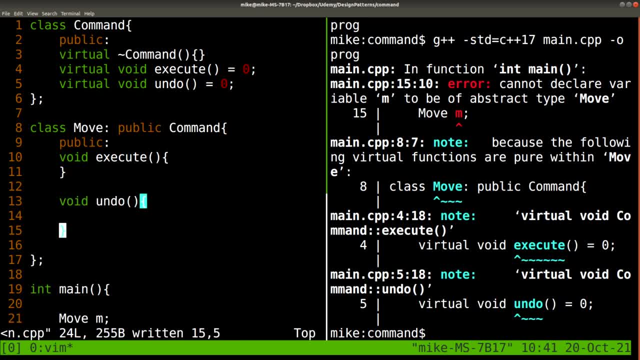 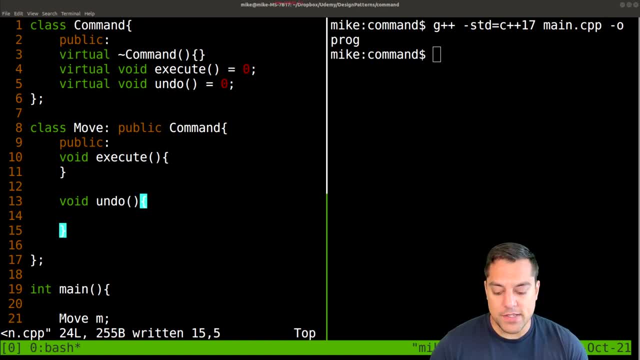 Okay, so let's try to rebuild this And for this time it compiles. Okay, and I still have my move here. So again, when I'm developing these commands, I like to move in very small steps, as small as possible, in order to understand what's going on. So if you're a beginner in 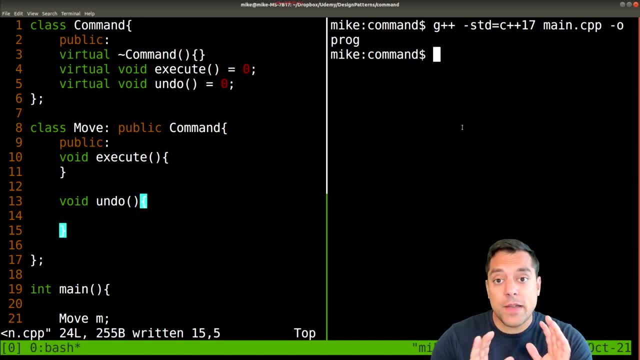 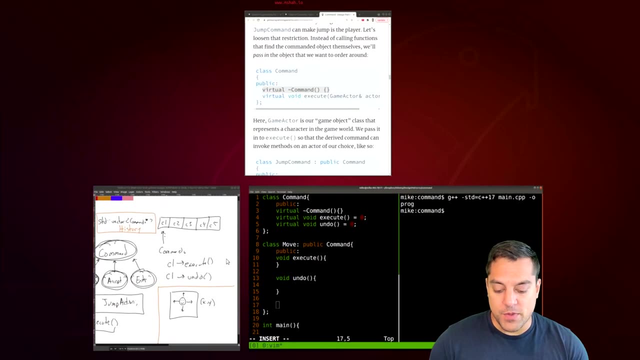 these design patterns. that can be very useful. Okay, so now that we have our program compiling, let's actually do something interesting, right? The goal of the move command was to set the x and the y position to something new. right, we're supposed to move our little. 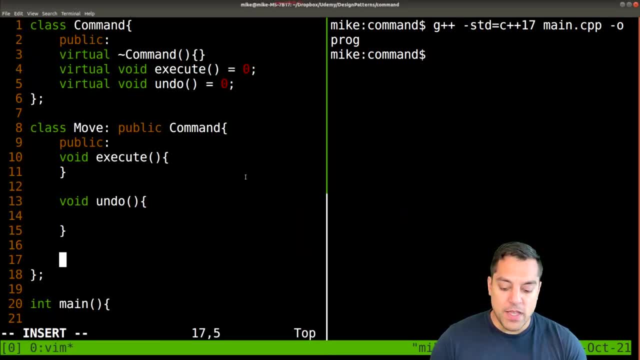 character around one one way or the other. Okay, so how should we do this? Well, part of our move action, for example, could be to set the position. Okay, so what are we setting the position up? Well, We're gonna need some sort of character here that we're moving around here, So in the game, 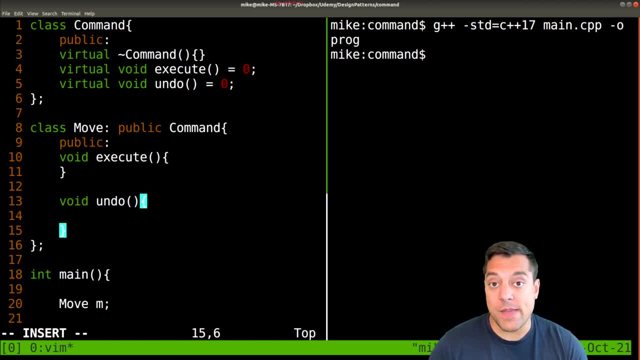 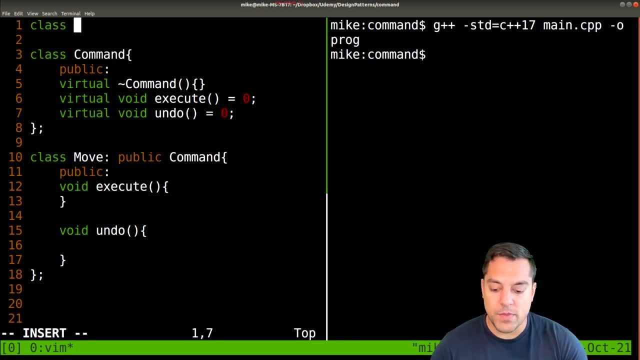 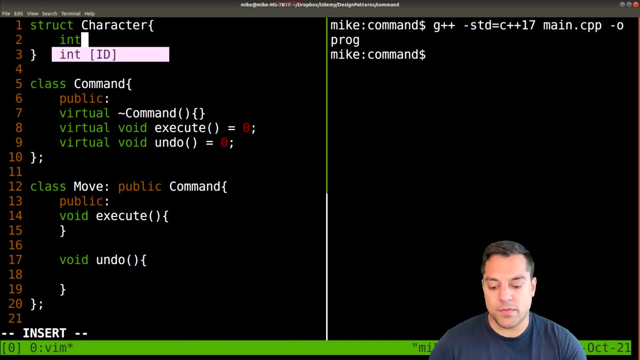 programming patterns book. they use an actor or some sort of game object. I'm just going to create another class here called the character, make it uppercase here And I'm just gonna actually make this struct and keep it really simple here. So they're gonna have an x position. 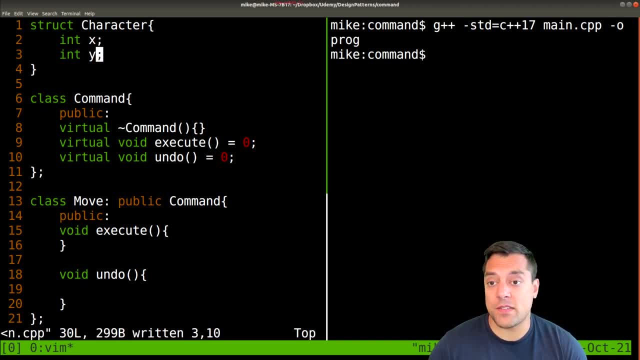 and a Y position. Okay, and that's what a character is. So now we do have a have to pass this around, which is fine here. So how do we want to pass this around? Well, as part of our- not our- destructor, excuse me, but part of our commands that execute for characters. 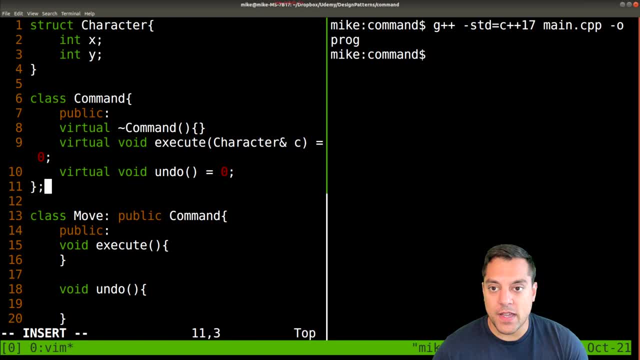 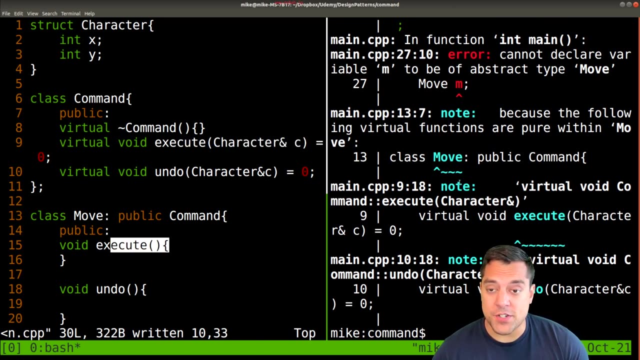 So we will have to pass this by reference here. So let's go ahead and do that here. So character C: And again, I'm just going to compile this so you can see that the errors that are again going to arise here, that we need to match our signature here, Okay, so that's always important that we do. 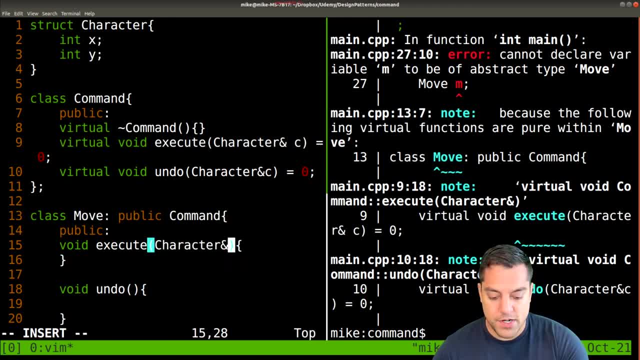 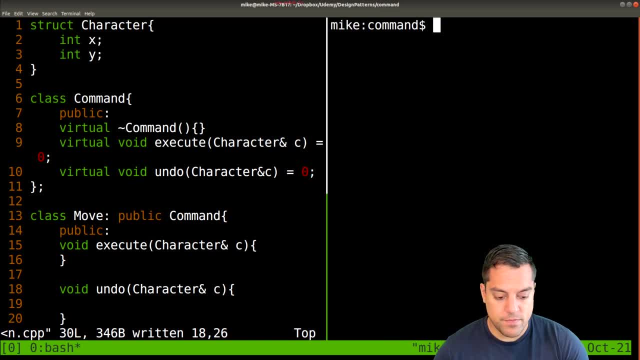 that And let's have our character here, See, okay, and our character that we're looking at, Okay. so now, if we recompile, just need to add a semicolon there And we're good to go, Okay, All. 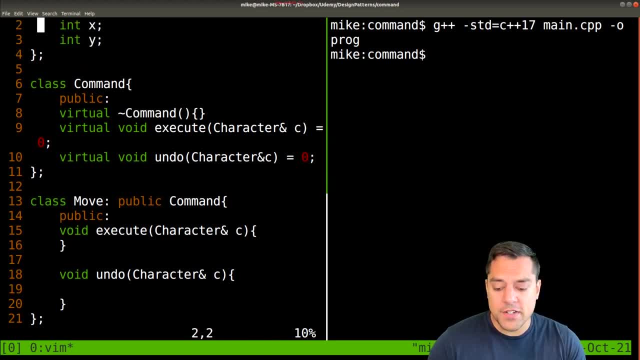 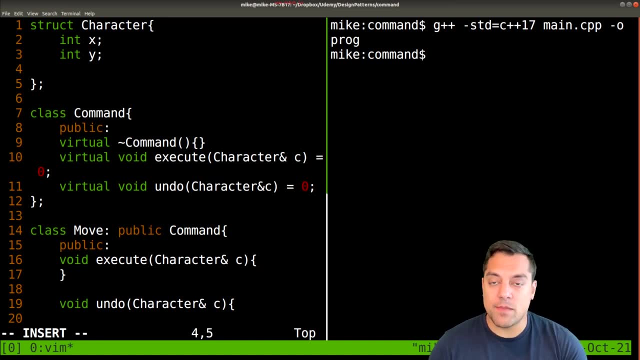 right. So now we have our category Character. they have an x and a y position and we can move them around, Okay, and we do want to do something more interesting like update their position, So maybe we have some function here for. 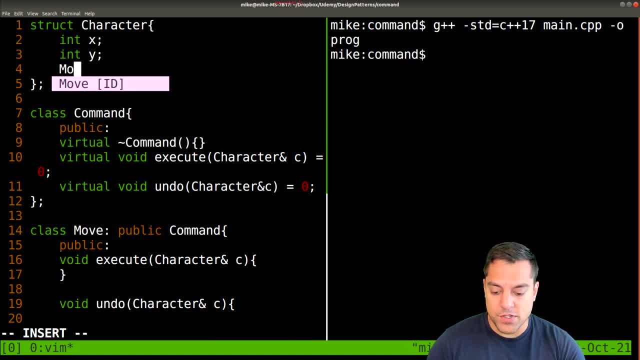 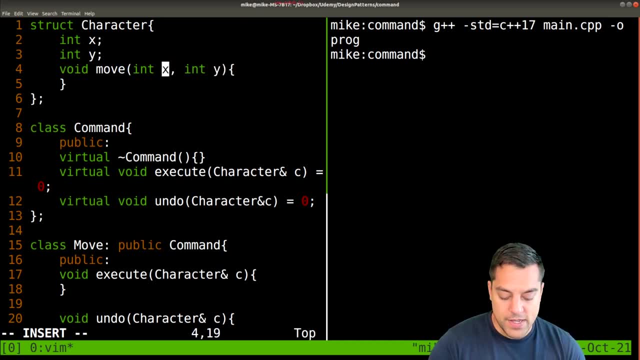 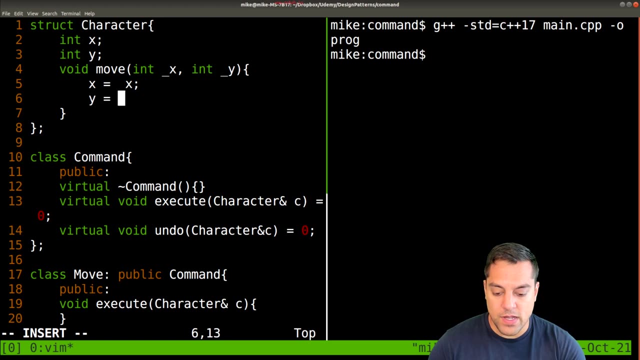 moving them, And we'll just call this void function: move and update their x and their y position here. Okay. so I might write this like this just for a little example: So x equals the x, Y equals whatever. the new y position is Okay, and then we update it as false. 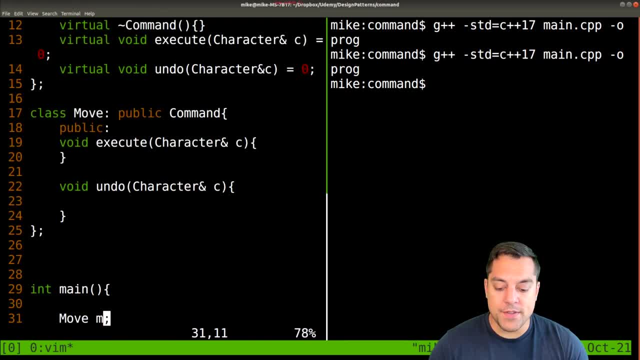 Okay. so now that we've got that compiled, let's go ahead and try to model what we're actually doing here. Okay, So let's just start by creating a character and creating some commands to move them around. Okay, and then we'll think a little bit about what we're going to do here. So let's. 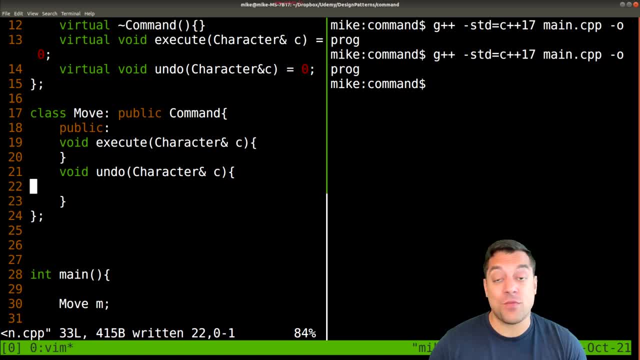 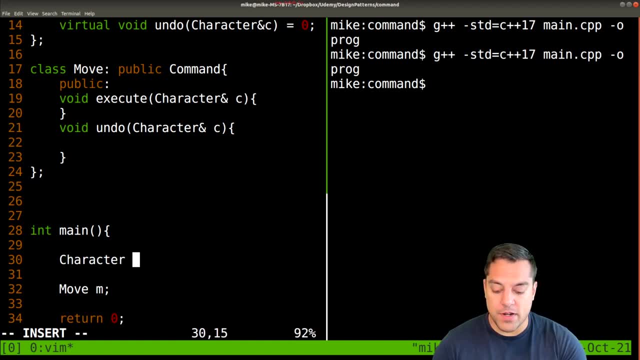 what is actually going on, execute undo And if we actually have enough here to execute our commands here, Okay. so we do need some character in our game here. I'm just gonna get a name, That's me, Mike, here, And maybe we want to do some moves here. Okay, we want to move and we want to execute. 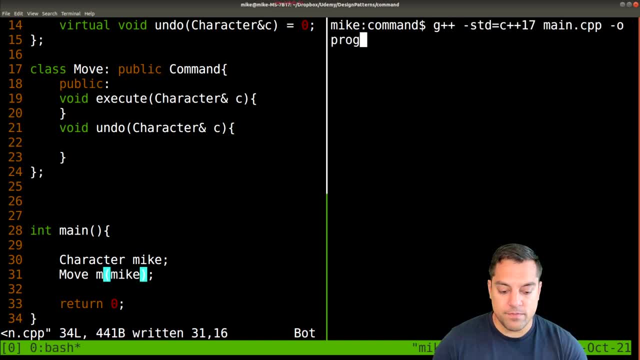 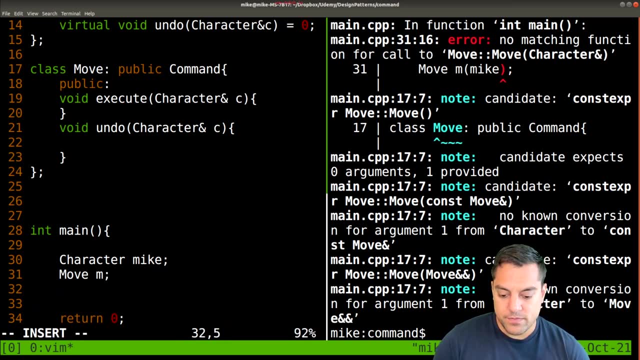 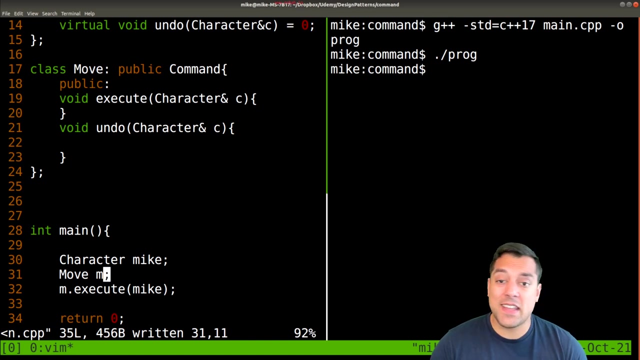 those moves on Mike, Okay, So let's see what's happening here, Oops. well, we don't want to construct this here, But rather we want to do our move and execute and take in a character- Mike as such- And let's go ahead and run our program here. Now, just to make this a little bit. 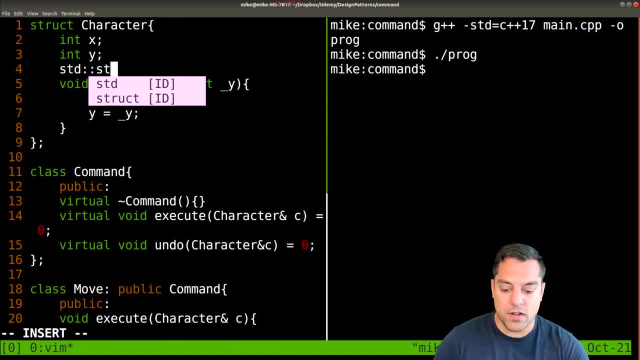 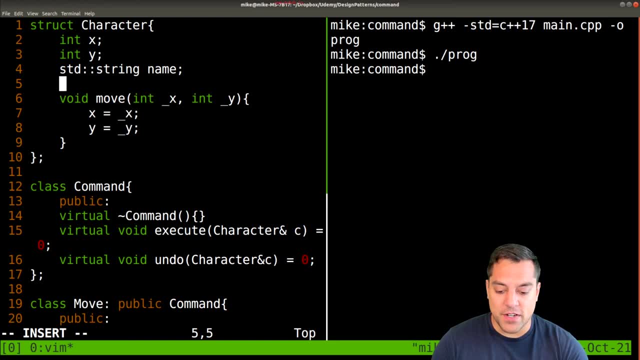 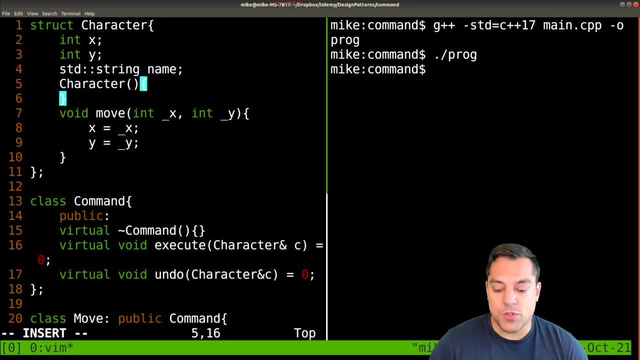 more interactive. I want to add just something else to our character class here a string and the same name of the character here, just to make it a little bit more interactive here. And that's going to mean I should probably have a constructor And I should probably have some sort of parameter here taking a string for the name. 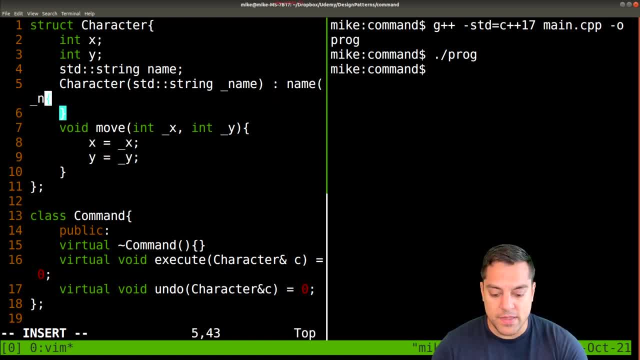 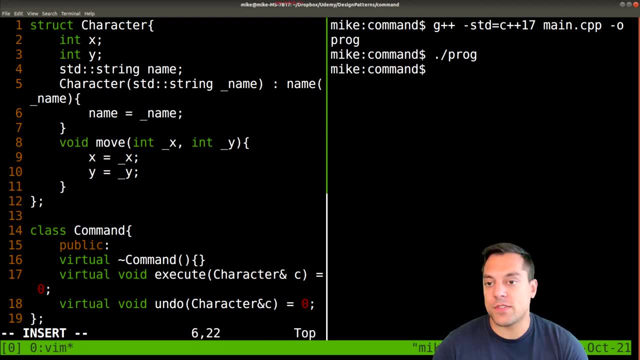 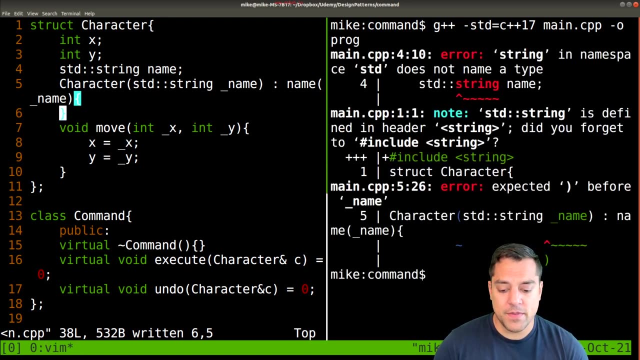 And I can do this in sort of the C++ way and make this a initializer list here. Some folks also prefer the style where you just do: name equals name, So it's super explicit. Either will work here. So now we've defined it. constructor, we should get an error here for our string type and 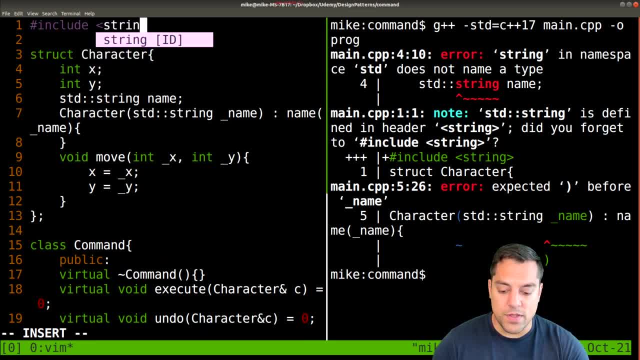 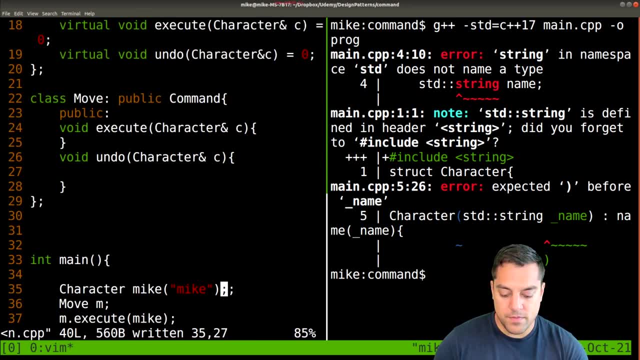 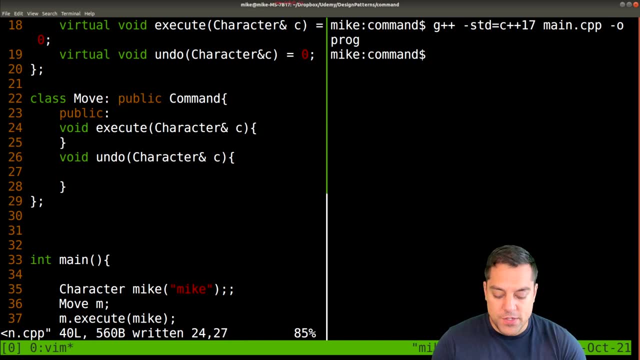 that we need to construct our object With the appropriate constructor here, So Mike and the character name Mike. So so far, so good here, Okay, and what we probably want to do here is, every time we move, maybe we just print out what 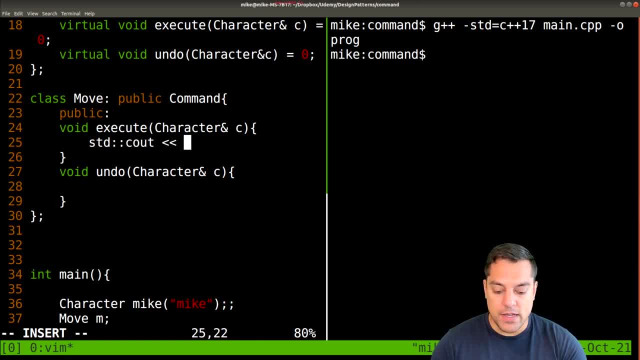 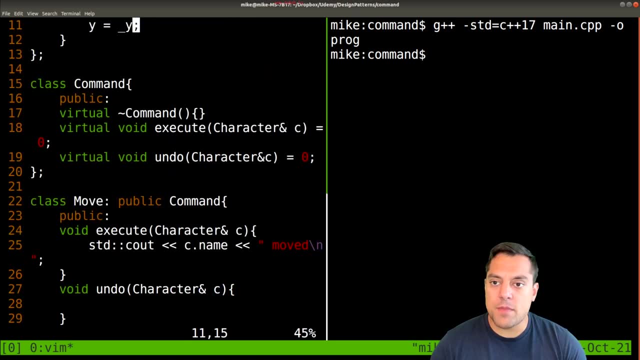 happens here. So let's do an output here. And C dot name space moved. Okay, and I'll put a little end line here, And I'm just doing this to confirm that the function doesn't do anything. So I'm just 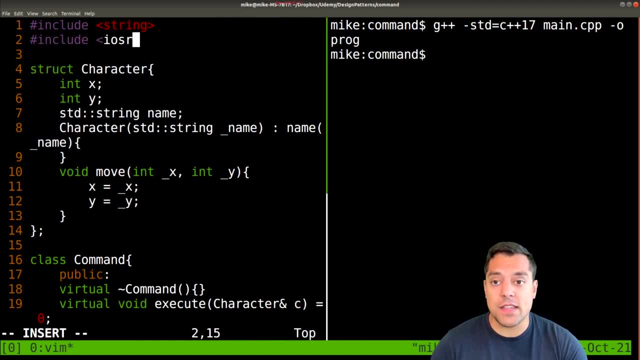 going to do an essay which is going to run this sequence, So that hasn't super messy right now And I that some action is in fact occurring on our character here. Okay, so I need to include the IO stream output library so that I can do some input output here, And I'm going to go ahead and 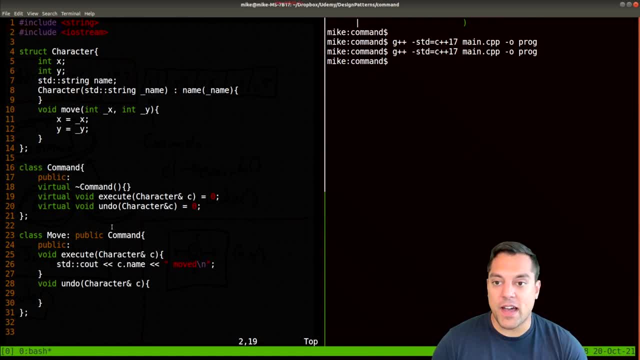 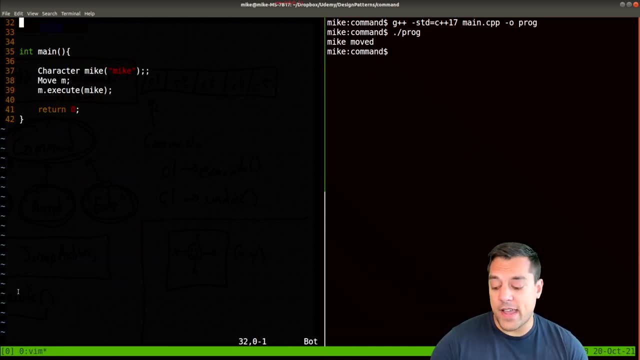 just reduce this just a little bit So you can see what's going on on the full program here. Okay, so let me recompile that, rerun it And we can see that our action in fact did occur here. we've created our character, we've got a type of command here and we have executed it. 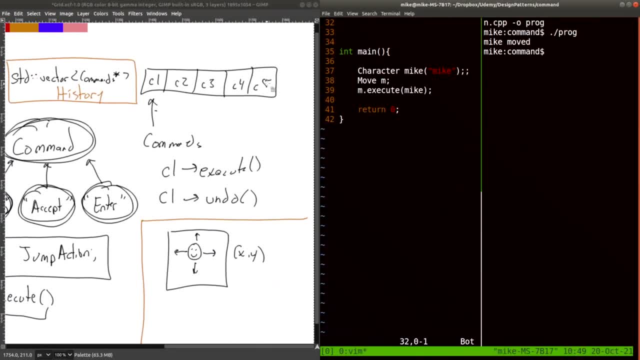 Okay, but again, let's push this a little bit further and see if we could maybe delay the execution here. Maybe let's do a series of commands and store them in some sort of data structure here, maybe a vector, for instance, a vector of commands, just to again. 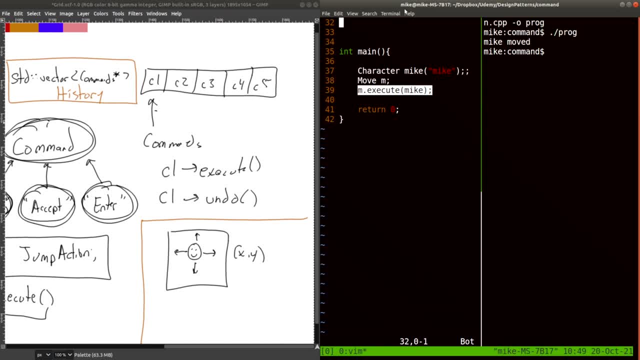 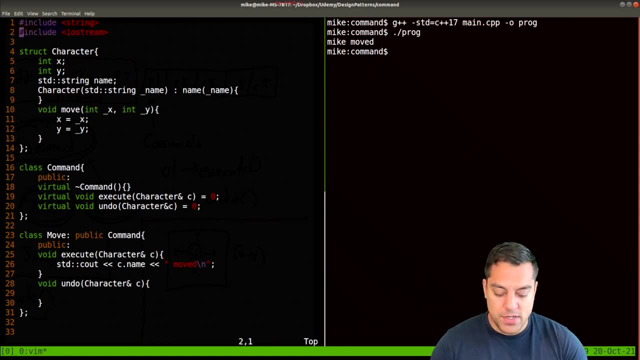 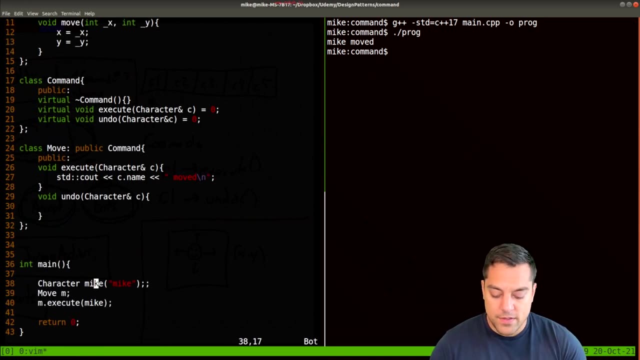 illustrate one of the use cases of the command pattern. Okay, so I'm going to need some sort of data structure for that. For now, I'm going to just do things here in a vector to start illustrating this, And let's go ahead and give ourselves. 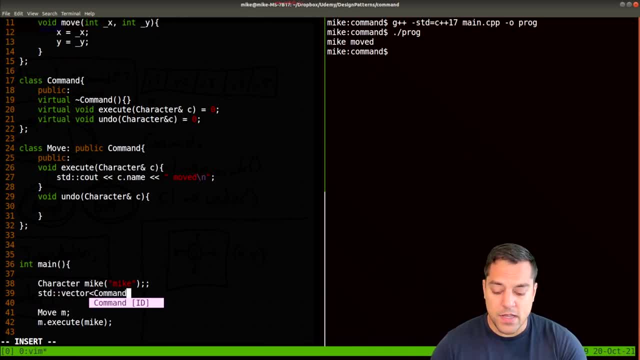 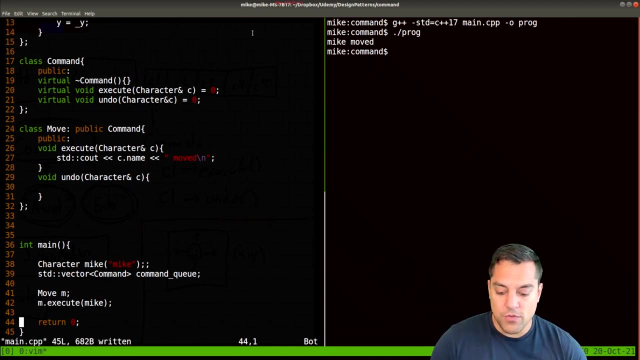 a vector And this is going to be of commands, And I'm just going to call it our command here. Okay, so every time that I create a move command here for our character, I want to enqueue that. So move one, And let's give ourselves a few. 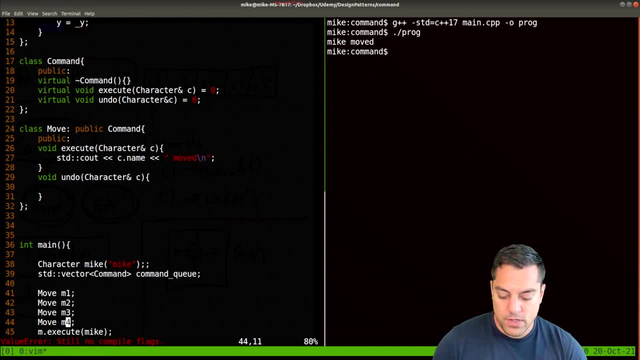 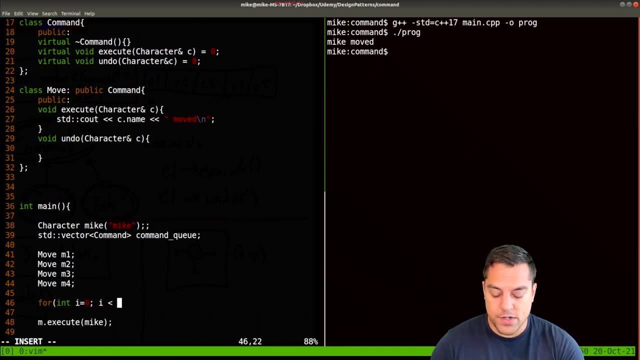 more moves here about four, And then we will just move through our command queue. So for int i equals zero, i less than man q. Actually, another better way, if I know that I want to iterate through, is to use a vector iterator. 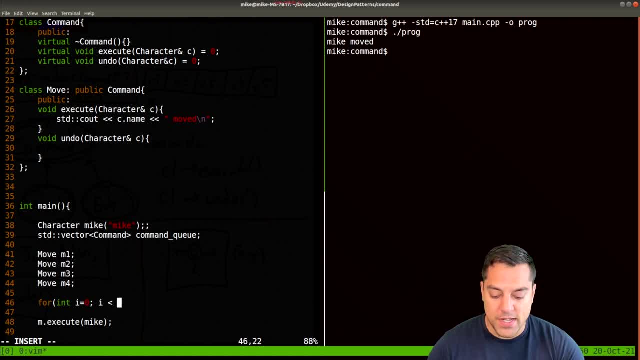 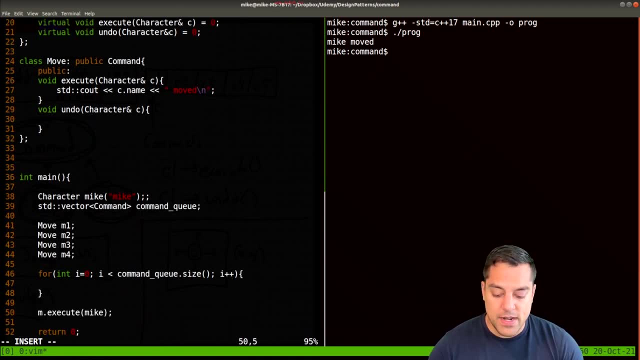 But I'm actually just going to iterate through these one at a time here. And q size: i plus, plus. And this time, instead of explicitly calling M dot execute, I'm going to be doing that on each of our command queues at index i. I'm going to execute these actions on my queue. Okay, so let's go ahead. 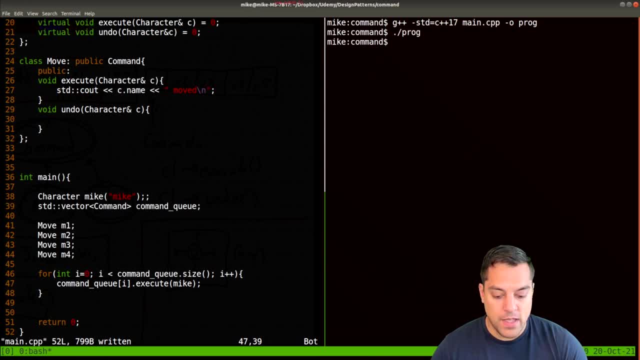 and compile looks like it's working here And I run our program. Okay, what happened here? Well, I haven't pushed anything into the queue, So I have to do that. Okay, so each of these commands, as I create them, I'm going to go ahead and enqueue them. 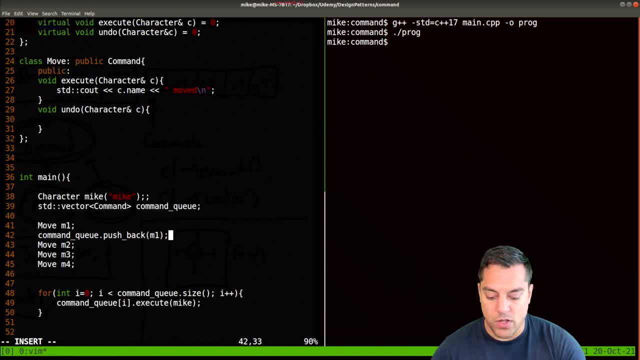 Command q: push back M one. okay, and repeat this Now again. this is a sort of slow way of doing it, But I'm just being very explicit. Usually, you're going to handle this by when you're doing this. you're going to handle this by when you're doing this� 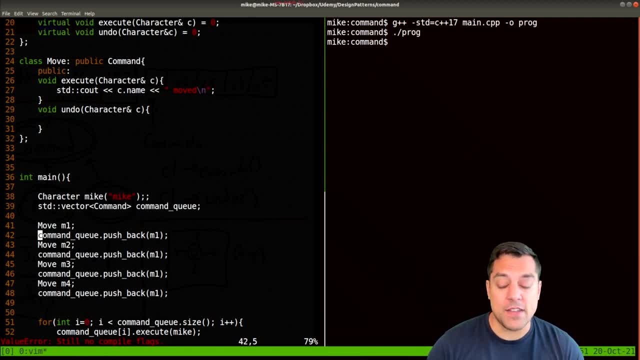 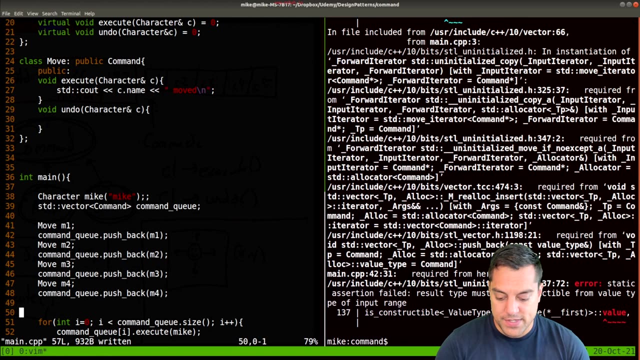 you press a mouse, click some command gets in cute, and then you maybe execute that command immediately, Or you can defer that action to happen later, which is what I'm choosing to do here for our moves. Okay, so let me go ahead and try to rebuild this. Oops, So we're getting quite. 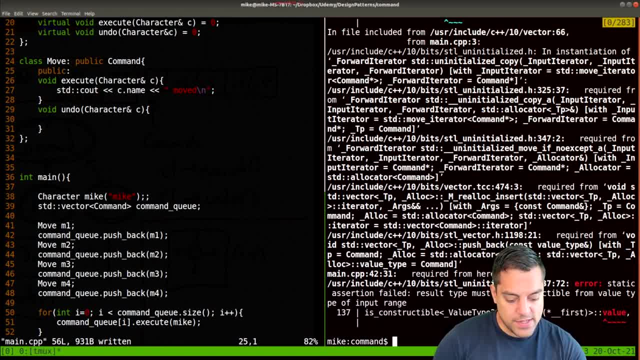 a number of errors here And it says: okay, static insertion failed. That doesn't quite like that. I'm just building this move commands on the stack and then just pushing those into our queue. So there are a few fixes here And this is probably how I actually want to model the command for this. 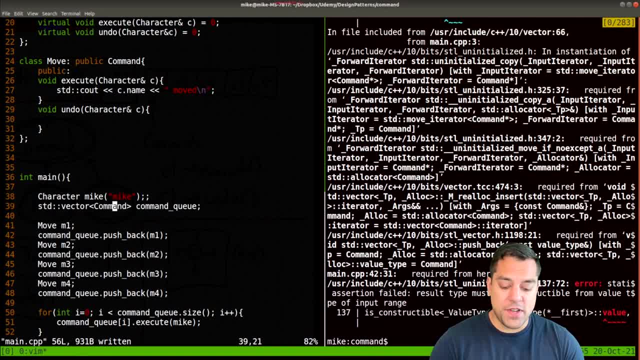 particular example, And what I likely want to do here is I actually want to store the pointers here Now why I'm doing this here, and let me go ahead and create each of these, And these are each going to be new moves, which are types of commands that we can store them in our vector again And just give me. 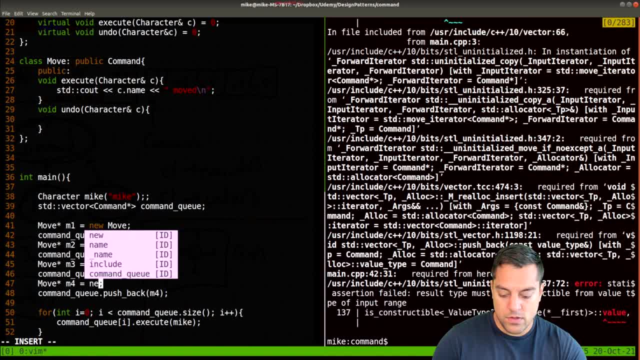 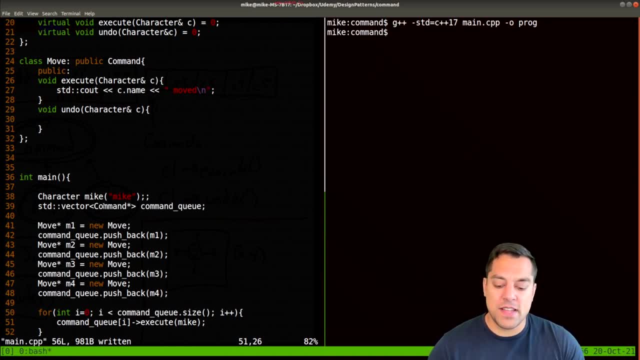 one moment here. new move, new move, And well, we are now need to execute as false. Okay, So what we're doing here- since we're essentially deferring or controlling the execution of the command here, depending on where this command is- is we're sort of responsible for managing the 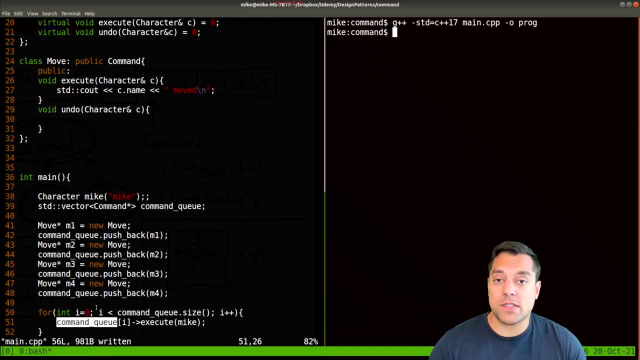 lifetime of our command. So eventually we do want to walk through this command queue and delete the commands. Now in this lesson I'm just going to show the raw pointers. you can make your life a little bit easier by using a smart pointer here so that it'll, when it goes out of scope, essentially 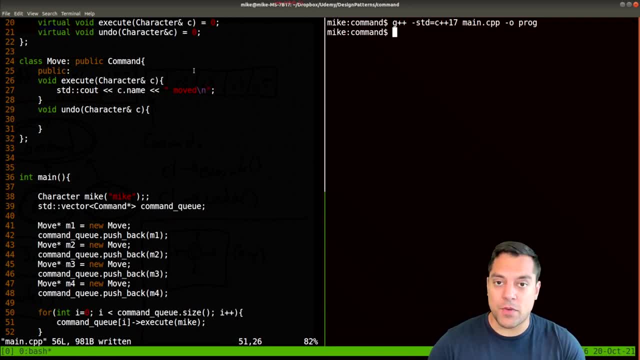 clean itself up. that's probably a safer thing to do, But I only want to introduce, you know, as few of things as possible here. Okay so, let's go ahead and do that. Okay so, let's go ahead and do that. 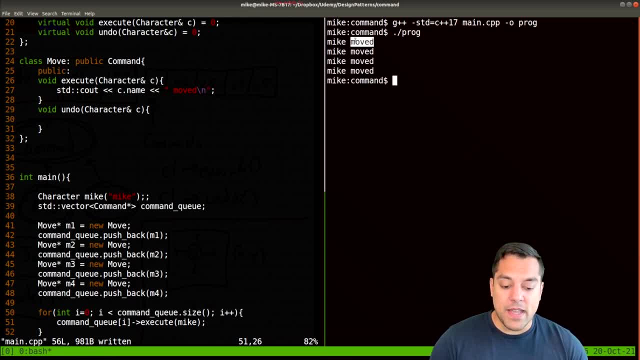 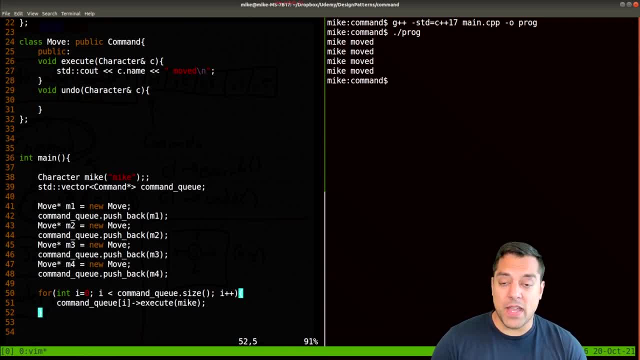 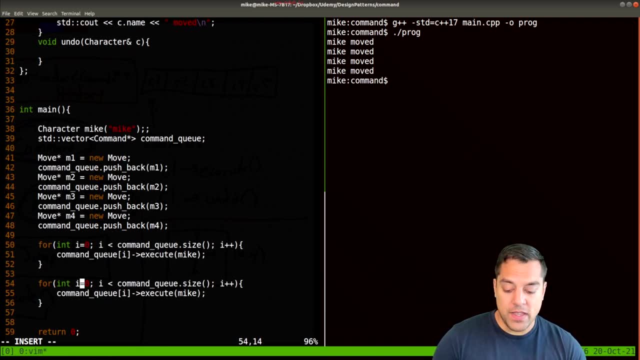 we're able to execute these commands. Okay. so what about the opposite here? What if I wanted to walk backwards through our queue? Again, you could use a reverse iterator for this, but I'm just going to take the size minus one- i is greater than negative one- And essentially walk backwards. 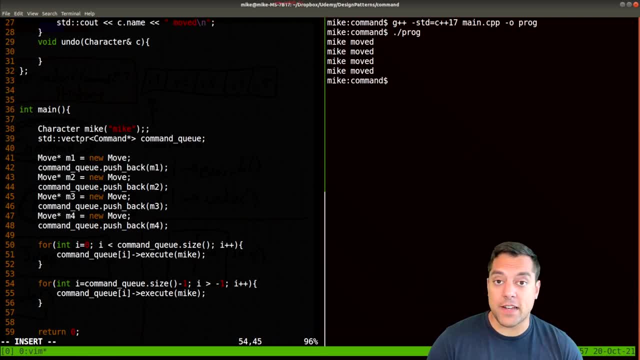 words through our what I'm calling our command queue, our vector data structure, essentially array. And let's see what happens when I undo on Mike here, Okay, And let me go ahead and execute this. And well, we don't have anything for undo, So let's go ahead and print out this little. 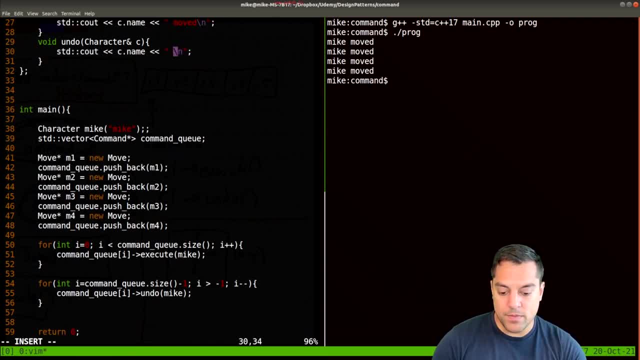 message to see if we are able to undo, undo, move. Okay, so go ahead and recompile, rerun, And now we can see that we are undoing four times, So we're executing on the same command. it's still in history that we're storing here in our vector. Now here's the question, though: how do we know? 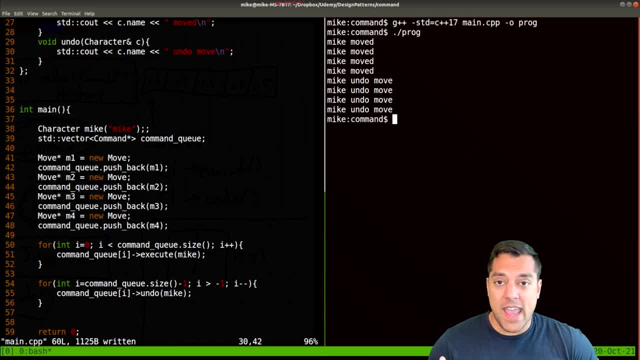 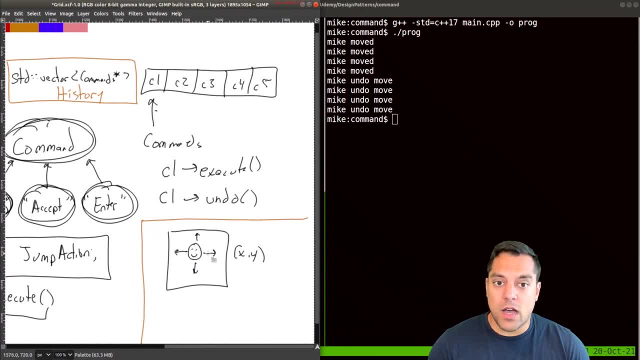 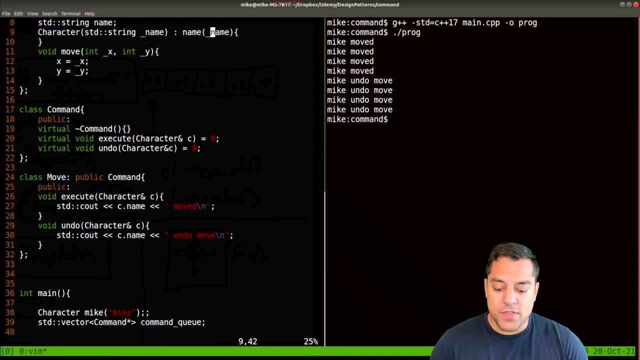 those. Where do I store that information? Well, the truth is, I need to store that information somewhere in my move command. So perhaps these could be private variable here And we have our character here And I could simply just do index and y And maybe, depending on what you want to do, 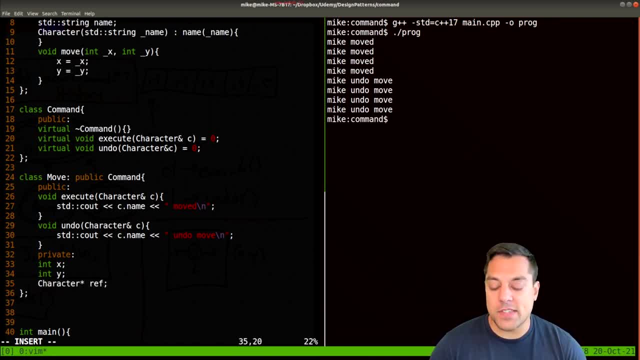 you might want to have a reference to this actual character here that you have, that you're executing the commands on Now again, this is where you can get in a little bit of trouble. So you might want to use something like a weak pointer, for example, to say: you know, maybe if I'm pointing to something, 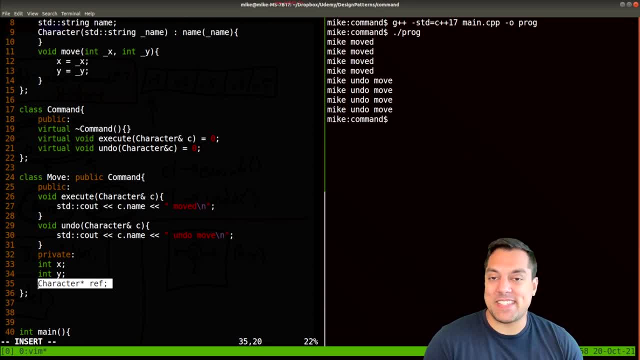 I can undo. it depends on your system here. for you advanced users who are watching this, Maybe a weak pointer is not strong enough, maybe you absolutely want to hold on to the reference, So you do need to think about that a little bit here. For simplification purposes, I'm just going to 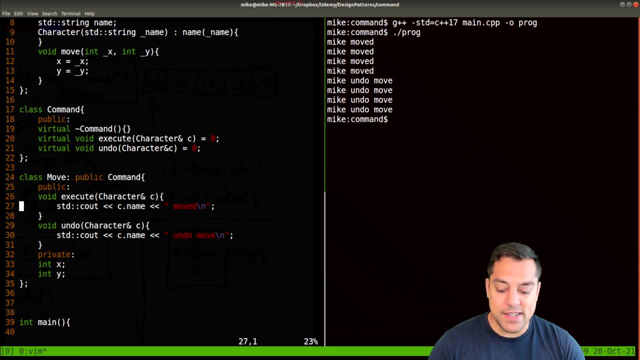 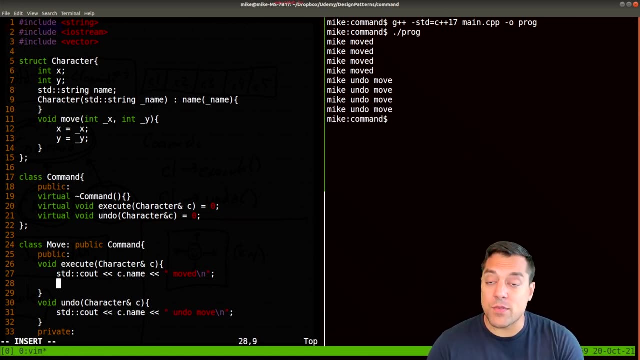 store the x and the y position here, So you can get the idea here that what we're doing is moving our character around. Okay, So part of our class here in our character is that we can move it around. Okay, so let's go ahead, And when we execute we want to do c dot move, You know. 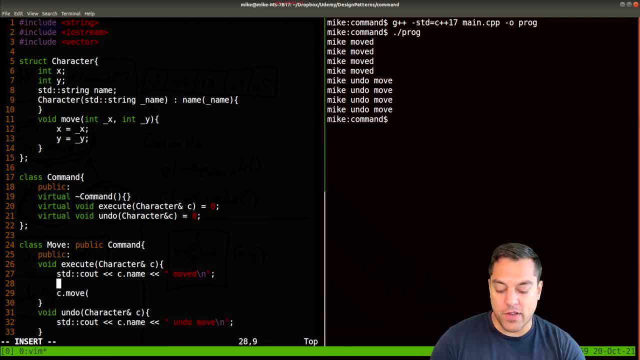 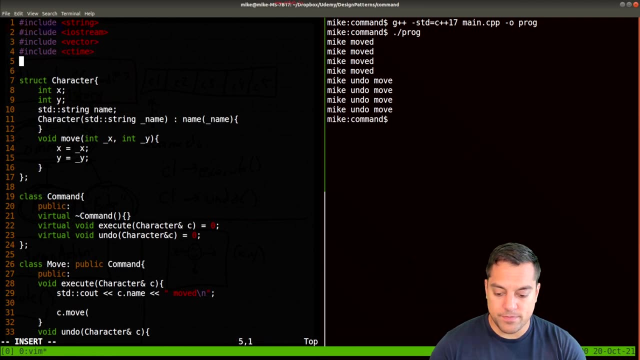 some random value. For now, we'll be fine here. Okay, so we need the random number generator And I'm just going to simply use the Rand functions here. So I need time, or c time, And the C standard lib, I believe. 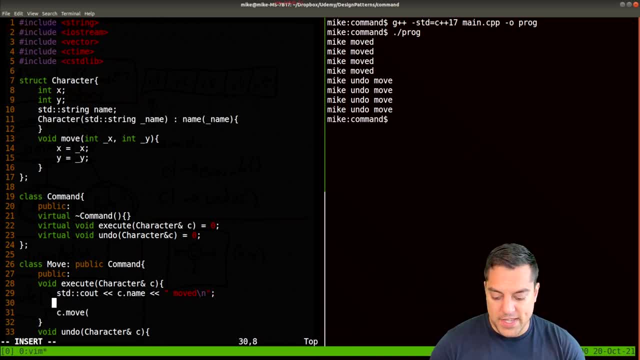 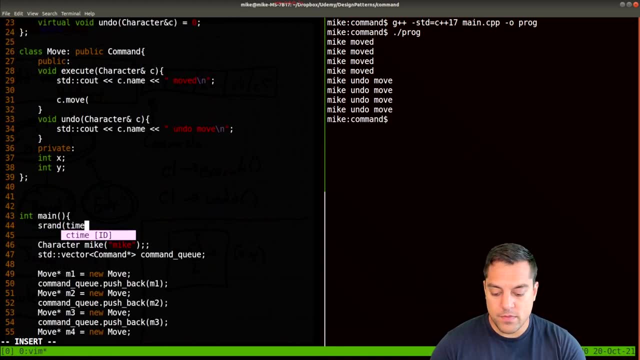 that's where these functions are. We'll know in a second if I'm right or wrong, And we should set up our random number generator here. This is the seed port And let's go ahead and just generate some random x and y positions. 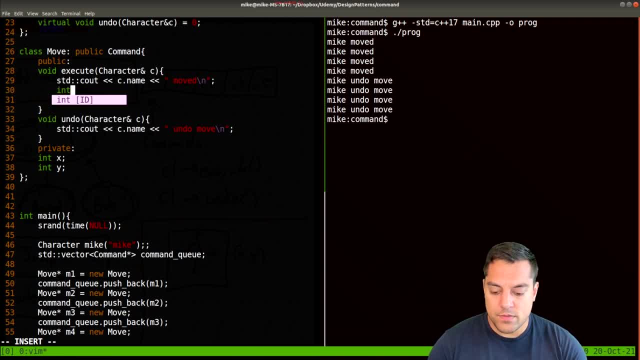 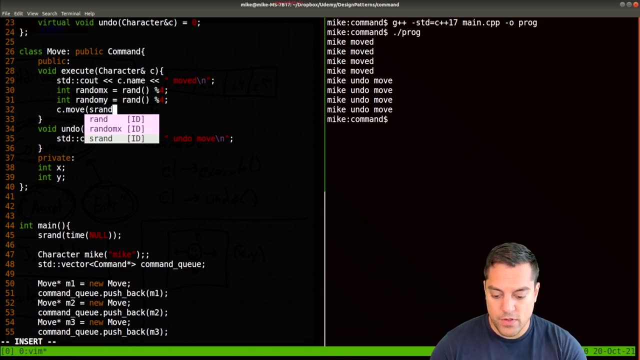 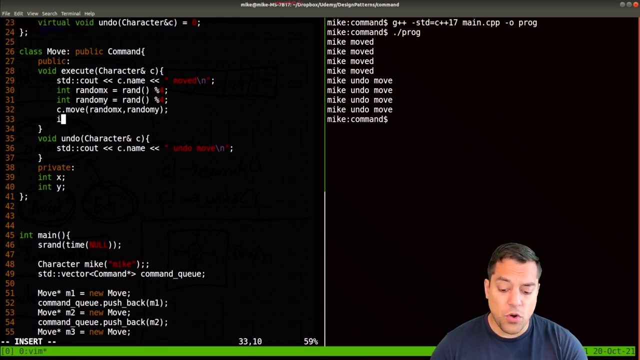 Okay, so let's go ahead and do it, And x is going to be a random value, say between one and four, something relatively constrained- a random y value- also the same- and we'll move a random x, any random Y value here. Okay, And what we want to do as well is store these positions: x, our random x and our. 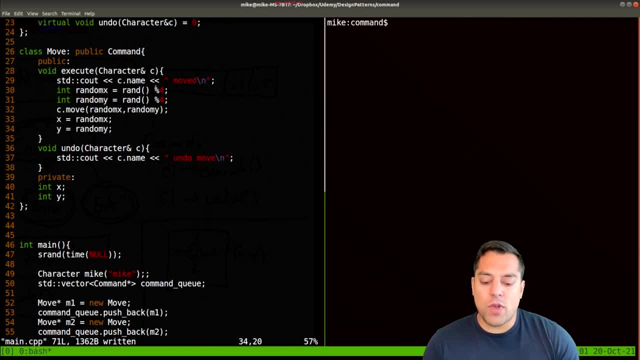 random Y position here, okay. So what I'm doing here is I'm able to, you know, generate some move. you know, the last action that I did is: well, I want to execute this move and move our character some random number between zero and three here, okay, and the x and the y position, And then I'm 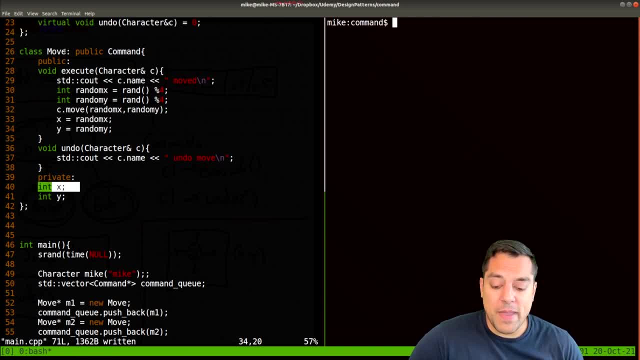 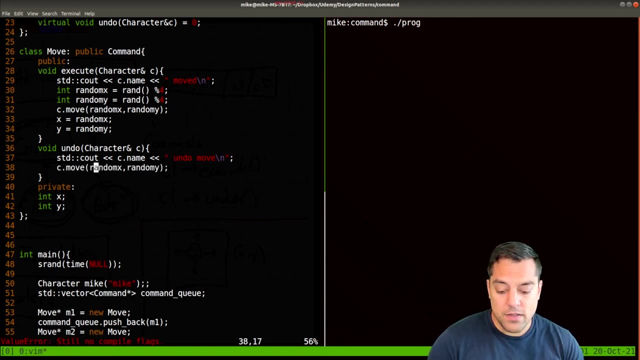 going to store that in the, the actual command here, the move command, as my x and y. So then when I'm undoing the command, I essentially want to do the inverse of this operation here. Okay, now what's the inverse going to be of this operation? while moving, but not the random. 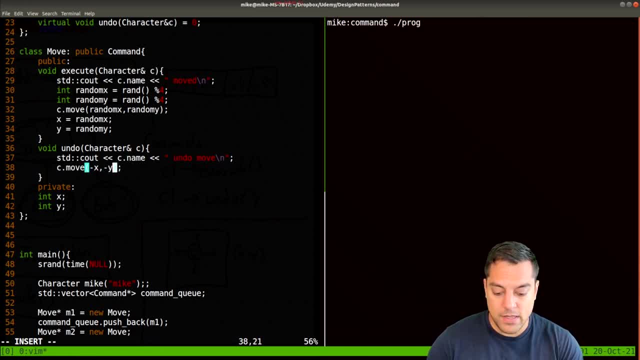 values, but the negative x and the negative y, And essentially that would put our character back to their previous position. So let's go ahead and make sure this compiles- Looks like everything compiled And in order for us to sort of debug this, let's update our cout statement So we can 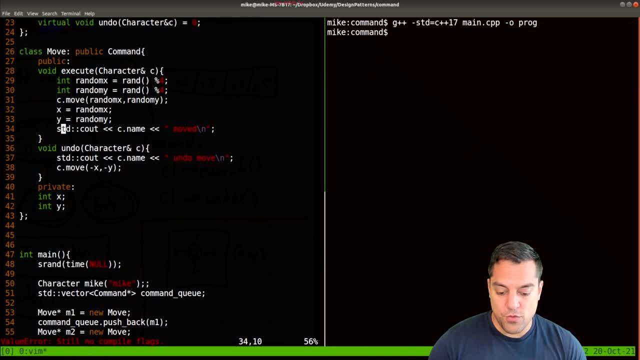 see where we have moved. Okay, so we've moved And I'm just going to update this to make the output a little bit easier on us, Because the x and the y, which is the same as our random x or random y values here that we're generating- 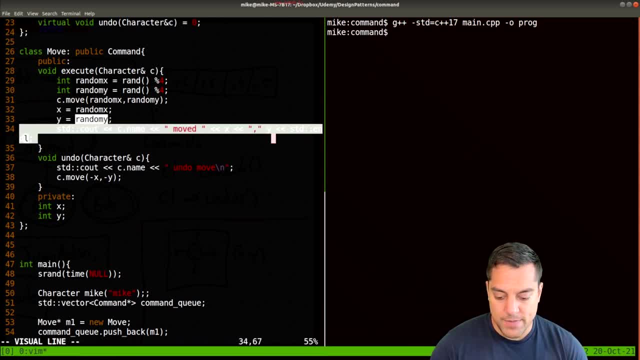 And we have a n line here And I'm going to copy this line here And I'll print out our undo here. I'm just gonna label this undo, Okay, and let me make this a little bit bigger So you can see it. 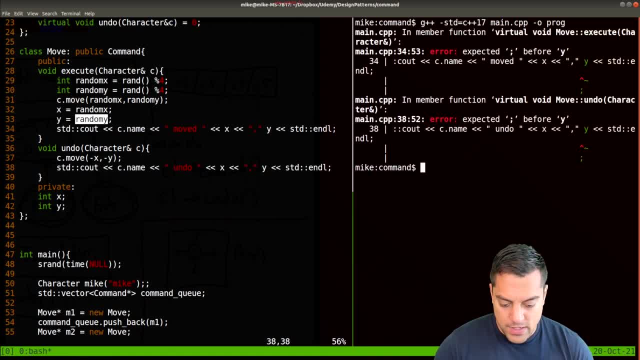 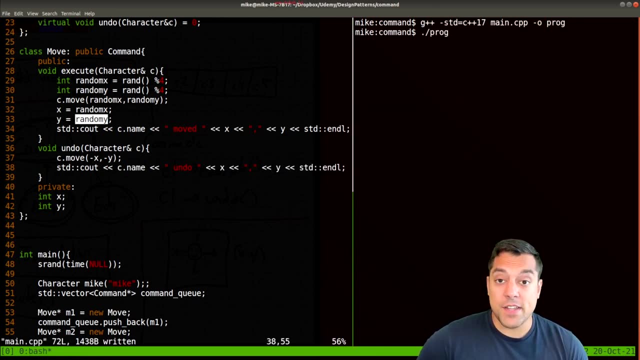 on one line here. Let's recompile. Whoops, one mistake, copy and paste error. So I'm going to have it twice, Or our arrows. Okay, And let's go ahead and see that it compiles, And let's go ahead and run. 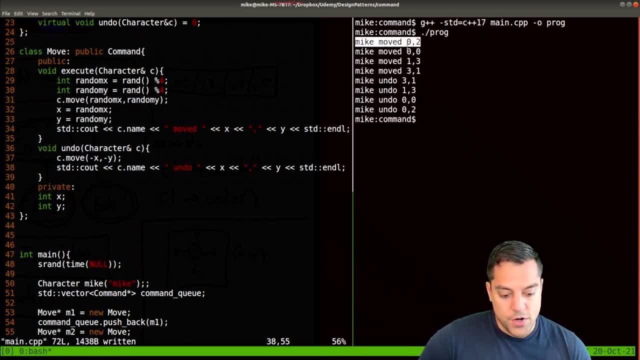 So the first move that Mike does is zero and two, then I don't move at all, Then I move one, three, then I move three, one. So the last action that I did here is to- oops, a little bit of a typo here. 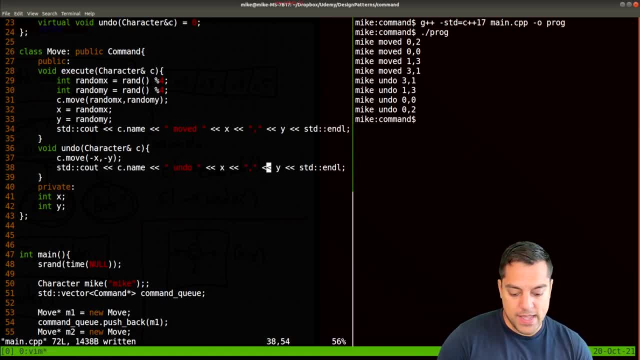 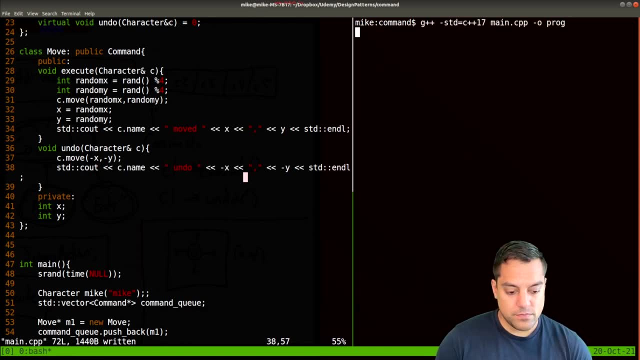 this is actually a negative value here, So let's go ahead and make sure we we print that out, But it looks like it is working here, Okay, so let me just rerun this again. So 32022110.. So that was my last move. So if I'm 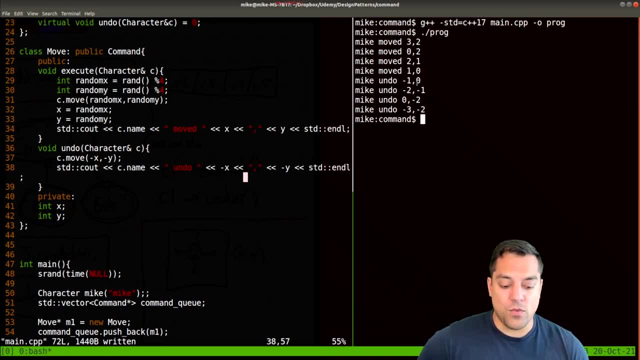 undoing the last thing that I did. I'm moving in negative 10. And then I'd move negative two. negative one. zero negative two negative three negative two here. Okay, And how I'm achieving that is well, I have my history of all my commands, just sequentially ordering them. 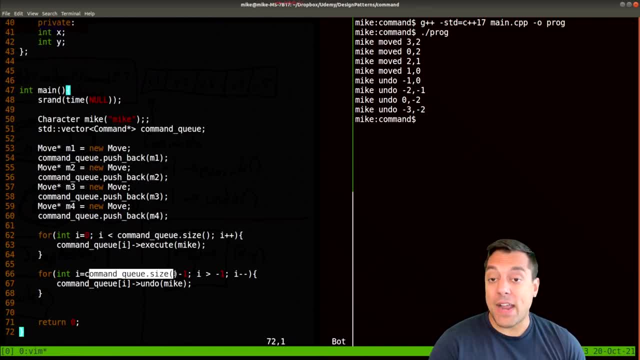 one after the other. And then, if I walk backwards from this data structure of vector, then we can undo our commands. Now, caveat, here there's probably a better data structure for walking backwards, And I'll give you a moment to think about that. So if you pause, 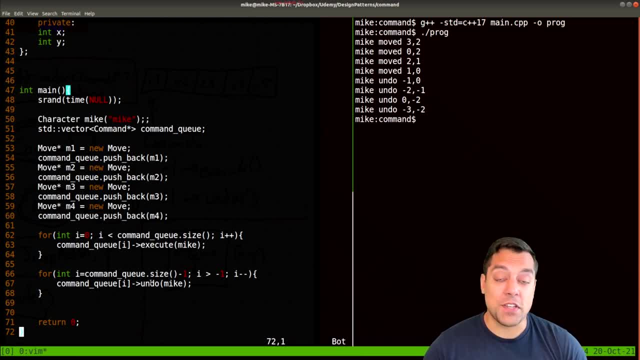 the video and thought about it for a moment. a stack is actually a really good data structure for maintaining your overall data structure. So I'm going to go ahead and do that And then I'm going to your actions. So that way, your last action is always on the top And then you can pop off the 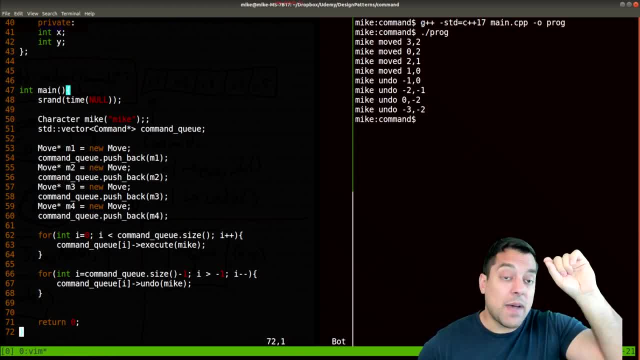 stack and undo that action, And you might actually pop off that command on your stack and move it into another stack. if you want to support a redo function which is essentially executing that command again, What command are you executing? Well, it's your move with the X and the Y. 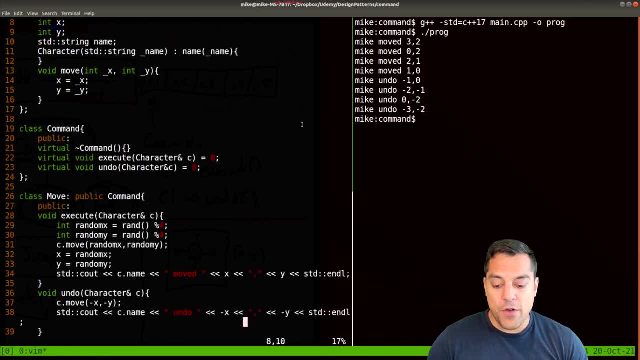 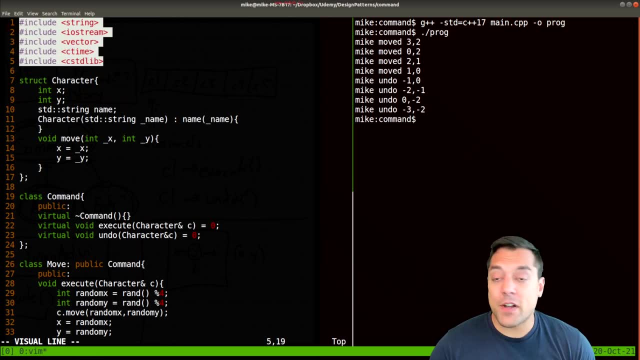 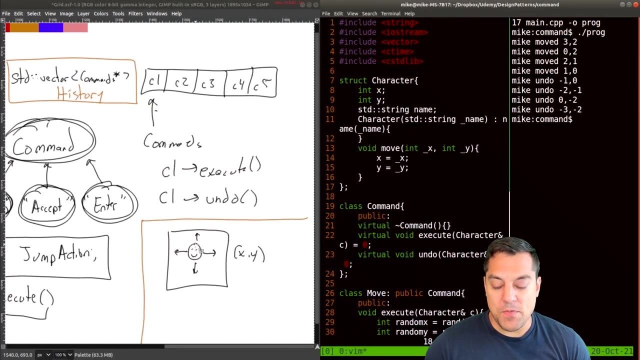 Okay, folks, so let me go ahead and just walk through this code one more time and wrap this up, because I think it's been a long enough video. So I've included some libraries to work with some data structures here, And I have a character here. That character was: you know this person here? 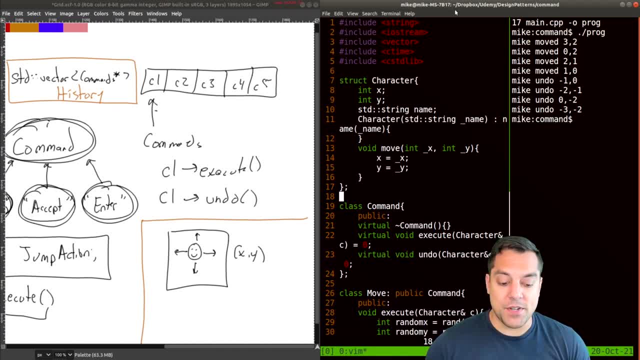 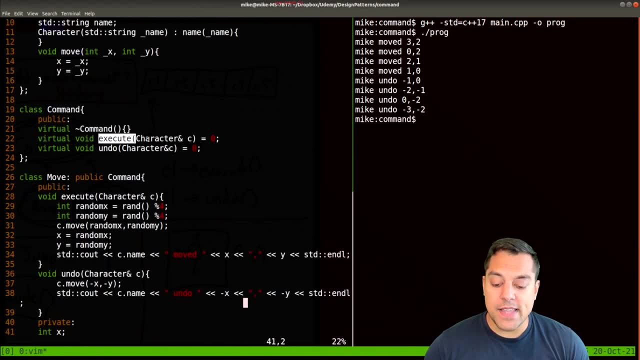 that we're moving on a map in some x and y position, And then we started implementing the command pattern here, And the important part with the pattern is that we have executed the as a pure function and undo as a pure virtual function as well, meaning that we must implement. 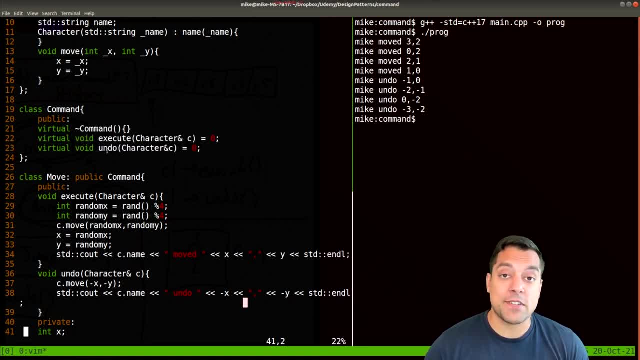 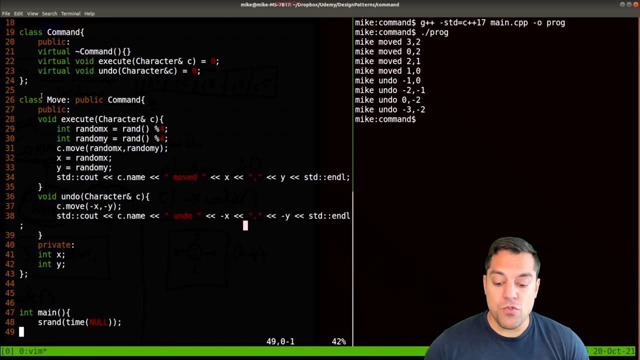 these, And the key is the execute and its inverse operation of undo, And then, when we want to model a command, we inherit from it. So move is a type of command, And then we perform our execute action and our undo, And we're careful to store the sort of state that we're modifying here, which is the 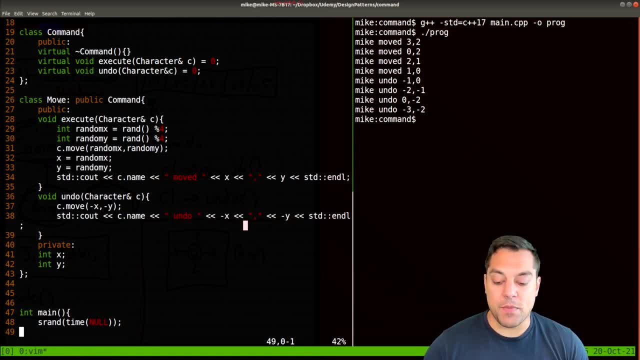 X and the Y positions for our particular execute command under move, which we can perform on different characters, And we had to think a little bit about what sort of data we're storing. Maybe if we want to store a reference to this character, meaning as a pointer or actually a reference type, we could do that as well. 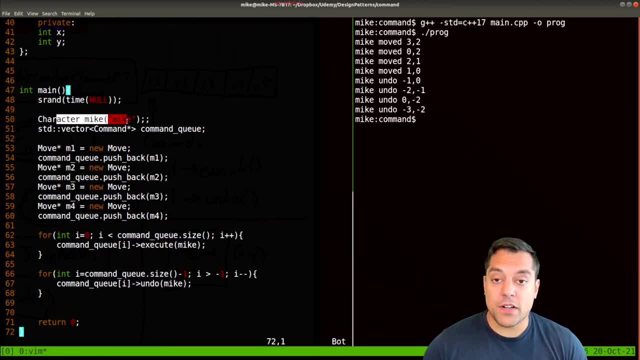 And then we did a little example. we set up our random number generator, created a character here and where we were going to store all of our commands. So this was the sort of command pattern. we're able to have our sort of callback or control where our functions are executed, by just pushing them into a command queue. 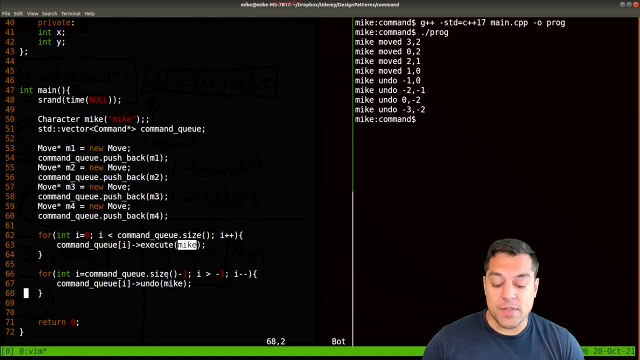 which is against the vector data structure, and execute those commands on a particular character. And we could actually execute these commands on different characters if we had different ones. Or maybe we could look at a series of commands that took place And maybe that has some meaning in our particular application. 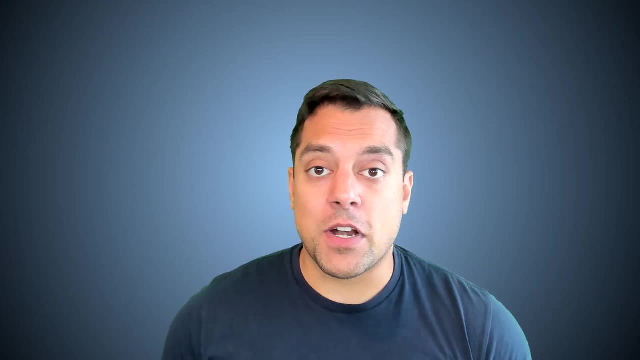 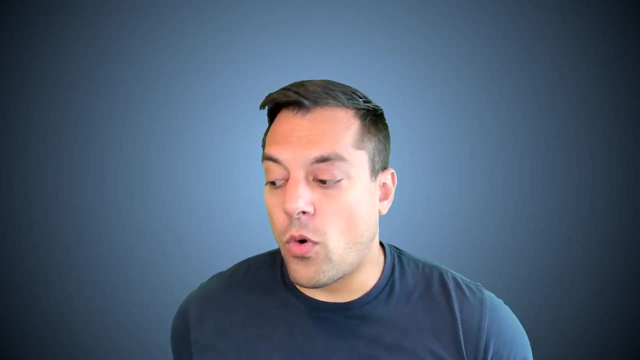 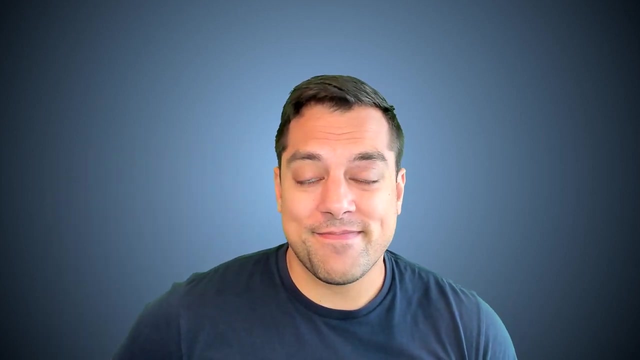 So I hope that this video has been helpful. If you have any questions, please feel free to email me at info at gmailcom, And I'll see you in the next video. Bye, This was a really useful video for you to learn about some of the design patterns. Take a look at some of the resources: the free book or get yourself a copy of the book or otherwise. the gang of four book otherwise is a good resource for folks working specifically in C++. So hopefully this was useful for the command pattern. If it was, please like and subscribe And we'll do some more design pattern videos in the future. Enjoy.